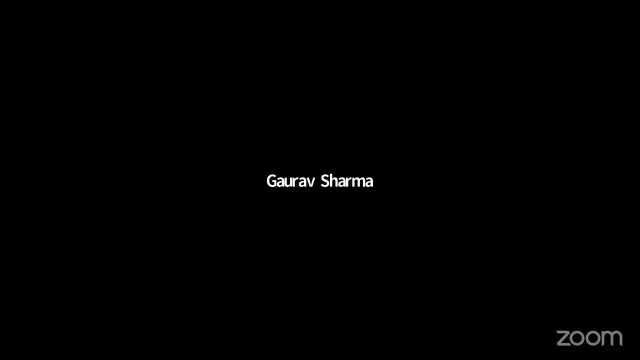 Thank you, Thank you. Today, this is just a demo class for you guys. So today we are going to discuss what are the topics that we are going to cover, And we will also check and cover how we can do the course of PCNSE. what is the path, how we will cover its topics. we will discuss all those things. 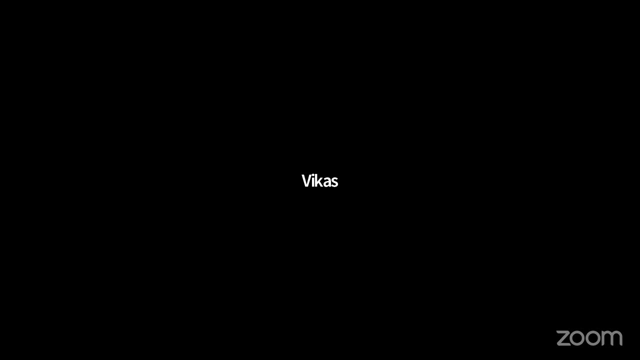 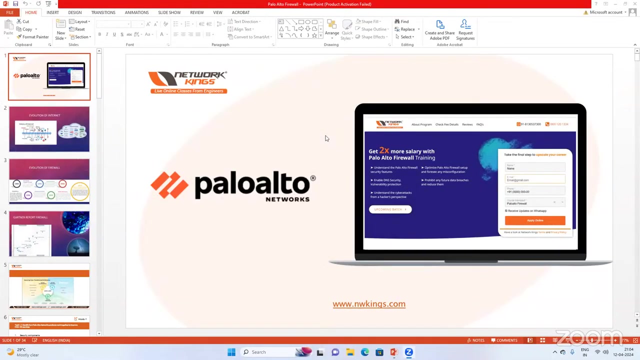 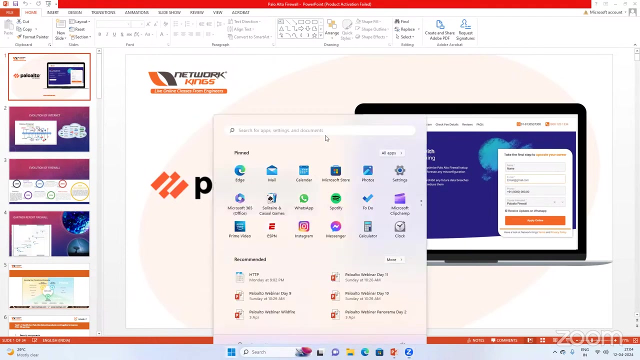 And we will also discuss a little bit about the company. So let me share my screen and then we can start up. Just give me a minute. So, guys, let me know once you see my screen. Yes, sir, Yes, Yes. 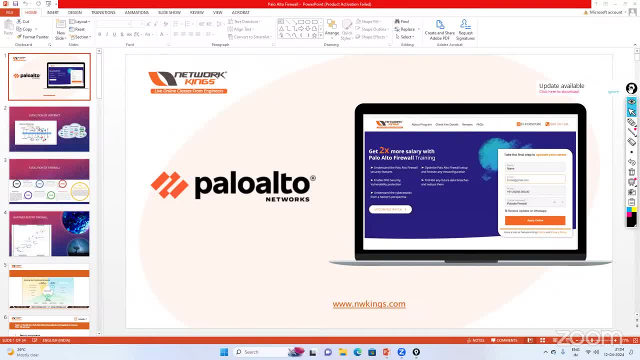 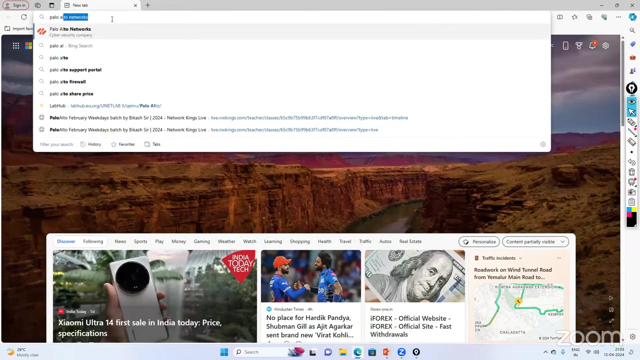 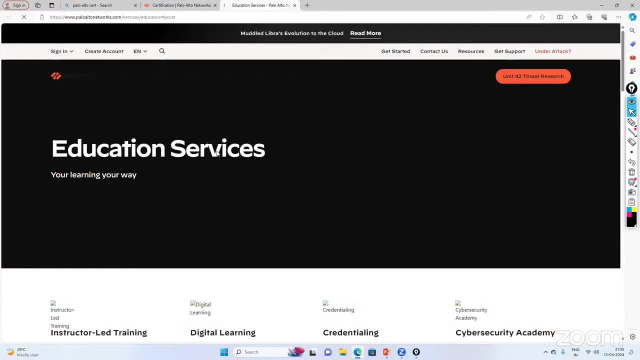 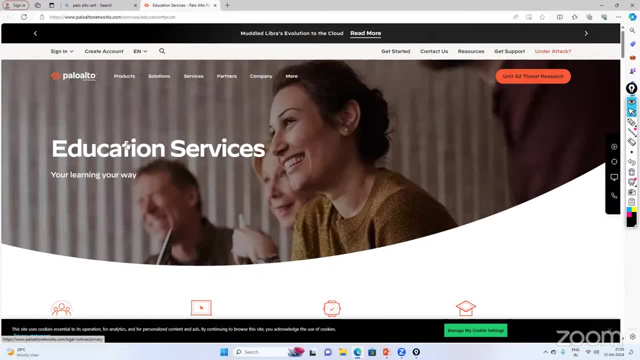 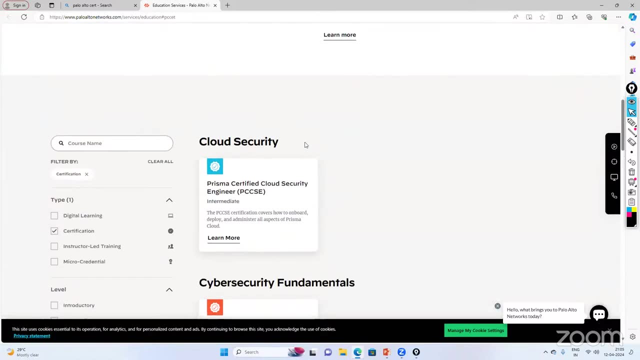 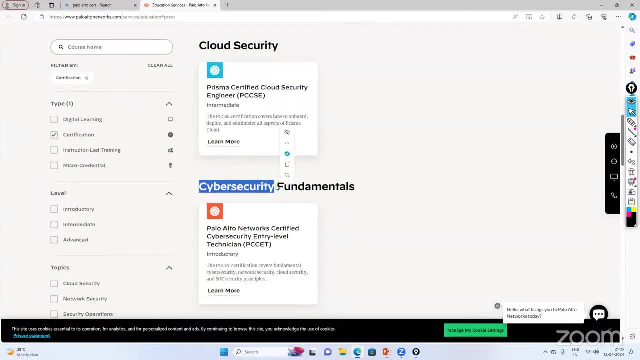 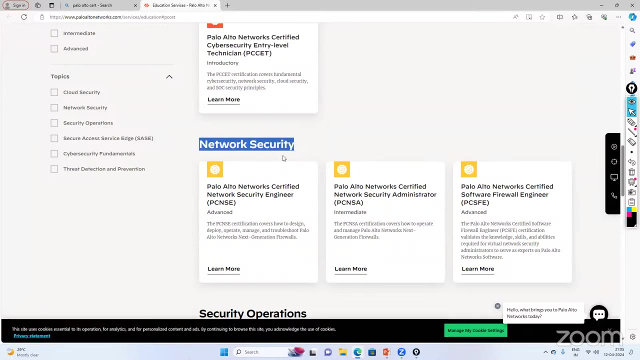 engineer, if you want to become a cyber security fundamental like, if you want to touch on the fundamental parts of it. so paulo paulo also has a certification which you can go through. our focus will be on network security, so we will focus on pcnsc. okay, pcnsc is our focus. 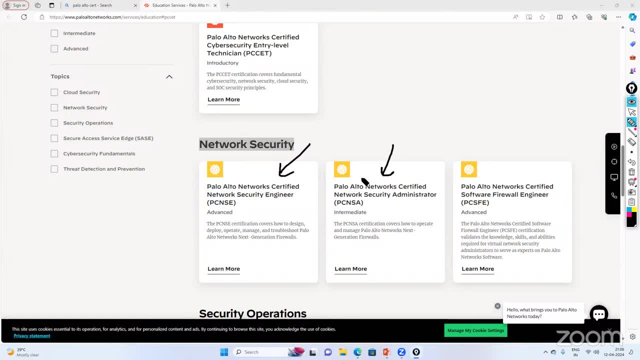 area, okay, and pcnsc basically this is an advanced topic. so in pcnsc we only cover firewall, okay, but in pcnsc we cover firewall plus panorama, plus troubleshooting, okay. so this is a little advanced topic. so there is no need that you have to do pcnsc. then only you can do pcnsc. you can take an. 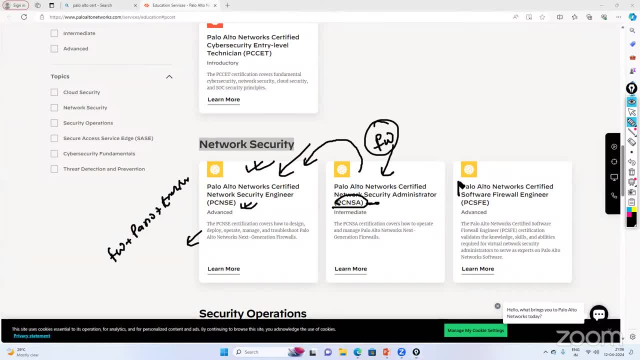 exam, there is no problem, okay. and the last certification is in network security on the cloud. so if you want to deploy firewall cloud, then what things, what technology and how they can do implementation. those software are taught in firewall engineer. okay, so good, so let's go on. goodbye. 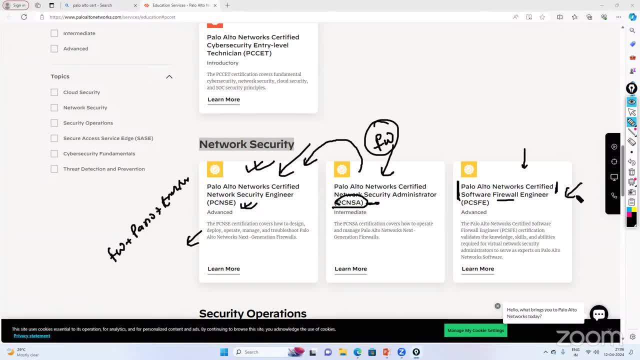 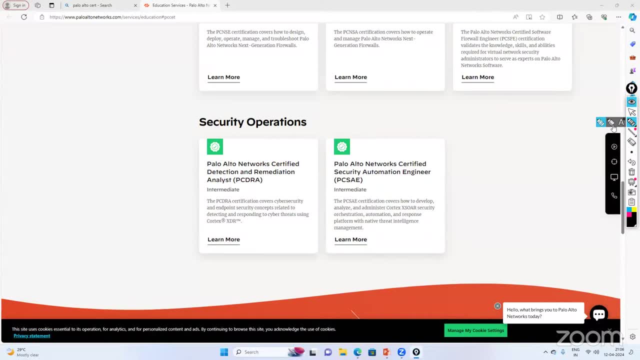 bye, bye Now. if you want to be an analyst in cyber security, you can do this certification. or else if you want to become an automation engineer, you can do this. So you have all the paths available. whatever, wherever you want to go, you can go with that particularly. 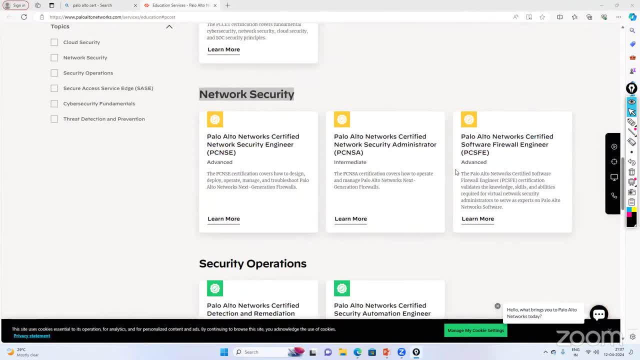 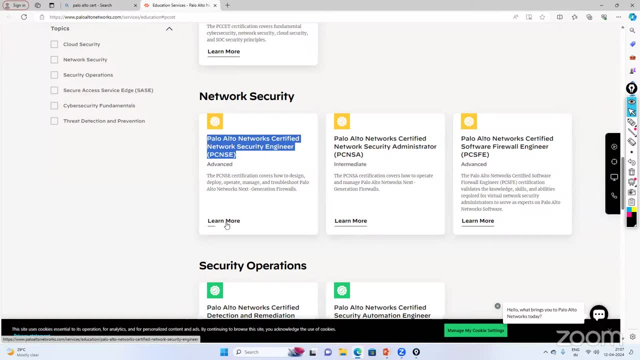 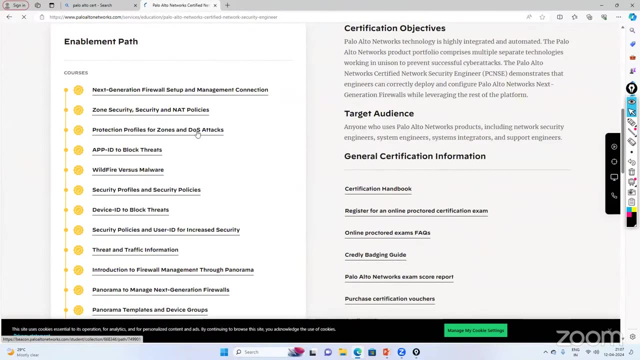 So this is the part of certification. So let's suppose, if I want to know about the Palo Alto PCNSE which we are going to cover, So let's click on learn more. Okay, And this will be our basically course structure of PCNSE. 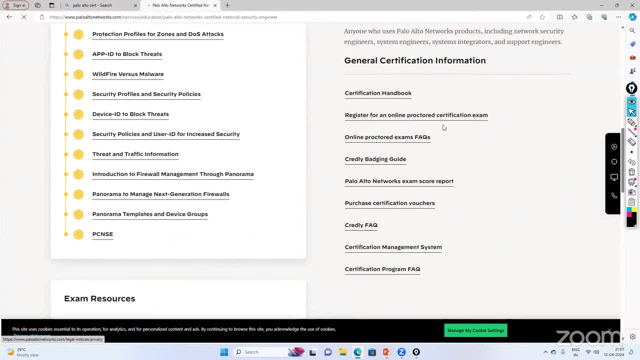 Okay, Here you will see some information of certifications, like some FAQ questions: when does it remain valid and you want to know about certification. So from here you will get that information, like how to do online, what is the process of proctor exam, what is the whole process. you will get all that information from here. 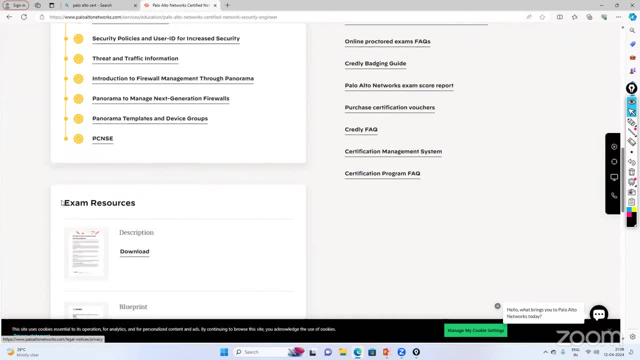 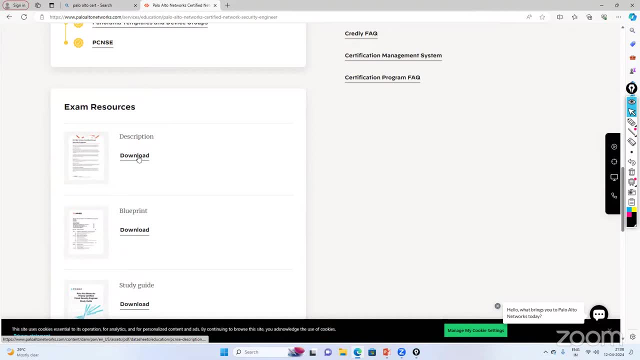 Okay, Exam resources means from where you can study. So this is your blueprint description. First, for whom this is basically targeted. for which engineers this PCNSE is targeted? What is the blueprint of this? What are the topics touched in this exam? 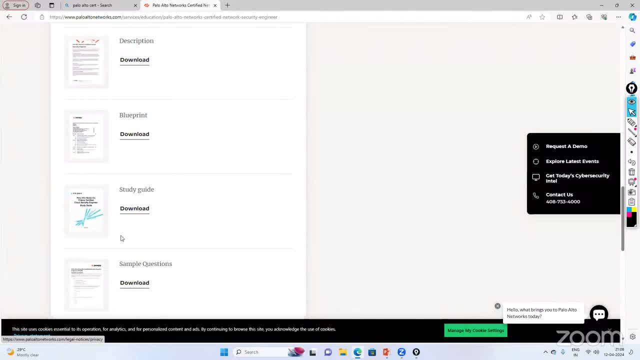 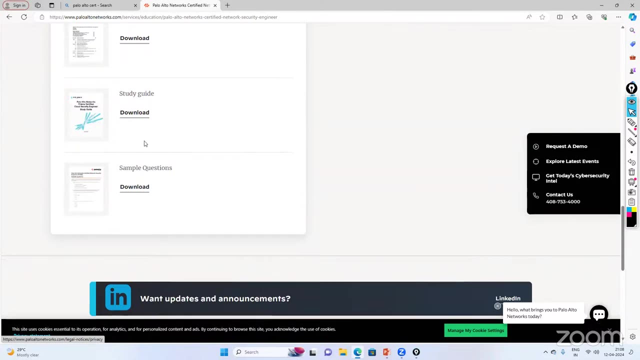 What is their study guide? Study guide is basically: what happens is that you are given some information about every topic. right That it is easy for you to study. Like if your exam is after 10 days, then you go through it once. then you will understand what topics we have to cover. like that. 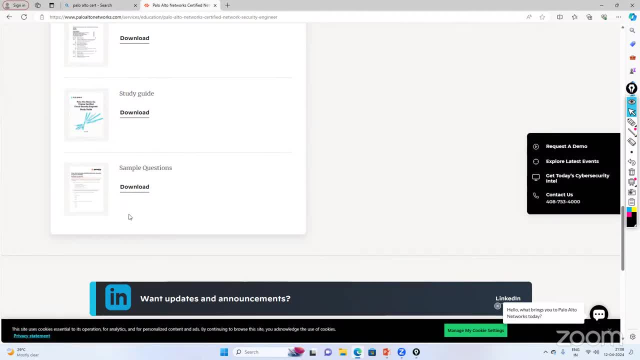 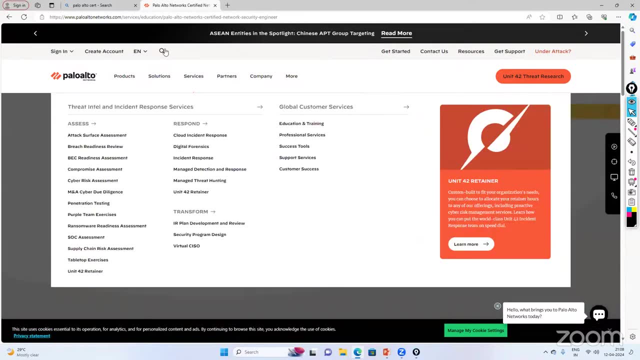 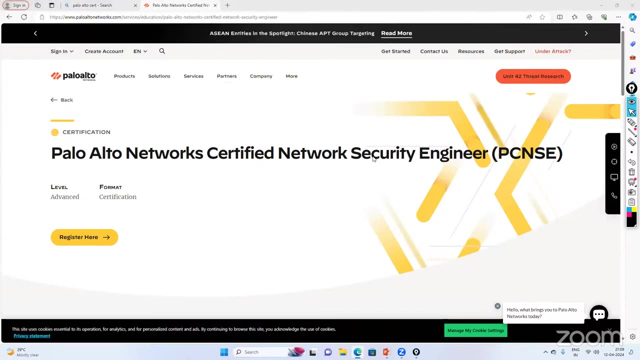 It has sample questions, So sample questions. So sample questions. come in the exam. you will get that here. So this is a very important website. If you want to visit it, then I will paste this link in the chat for you. you can bookmark it in your web browser. 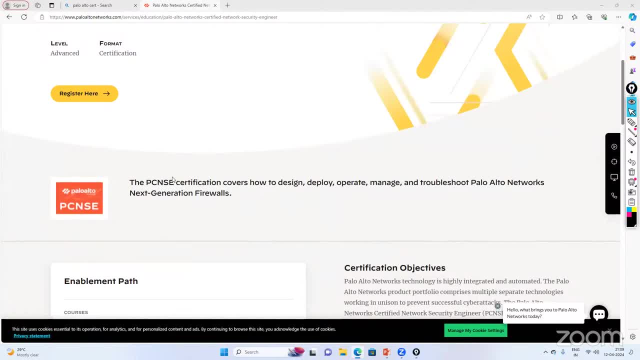 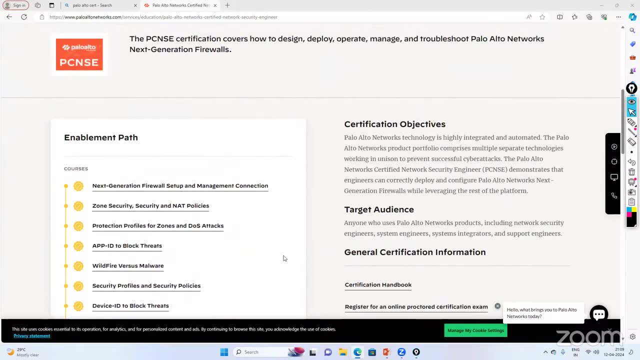 So it will help you basically to understand about this particular PCNSE course. Okay, So this is all about the course, guys. Okay, Now in this session we will see which topics we are covering. Okay, Because there are some topics which cannot be covered in the lab. 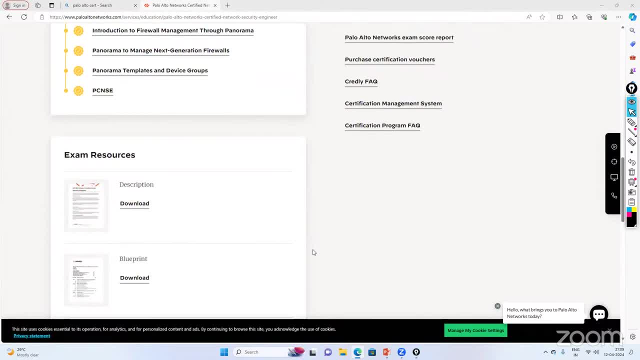 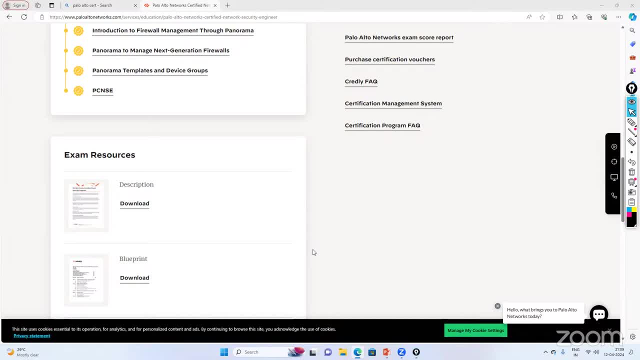 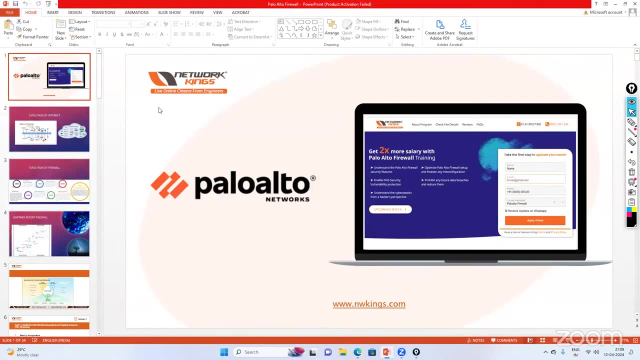 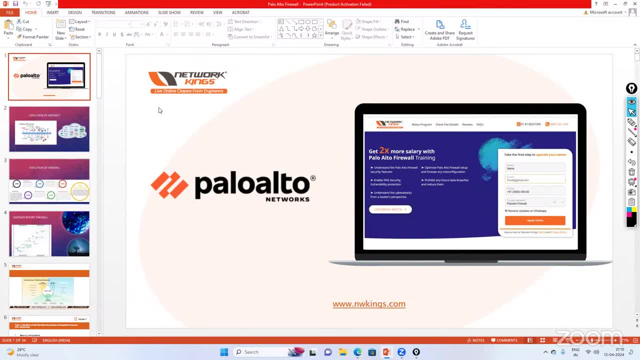 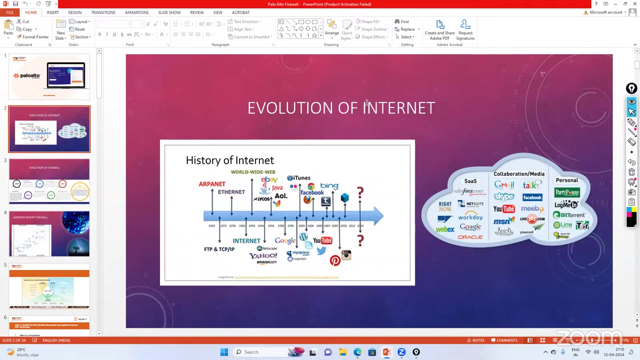 Okay, If you have any questions, then please ask me, Or else we will go further. Okay, So maybe towards the last. if you have any questions, let me know. okay now. so First of all, we understand the internet, that how the whole internet has grown from our history, and now how the internet is connected and where it is connected. 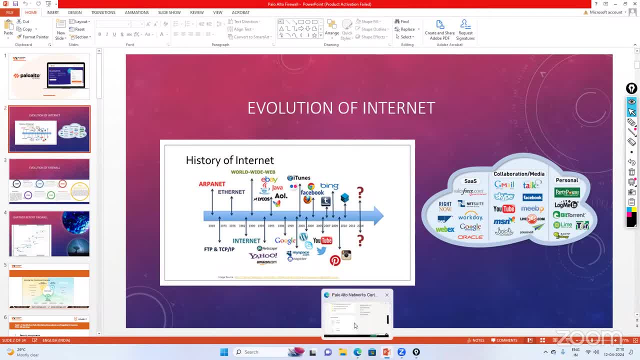 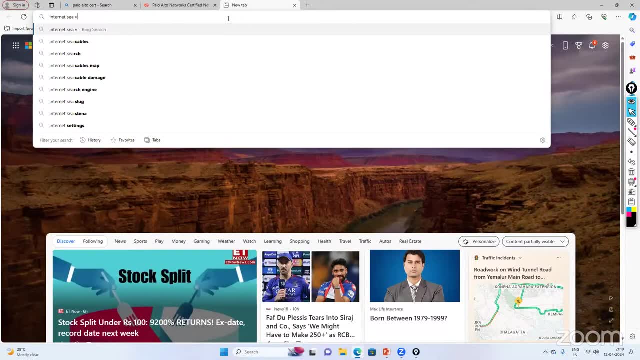 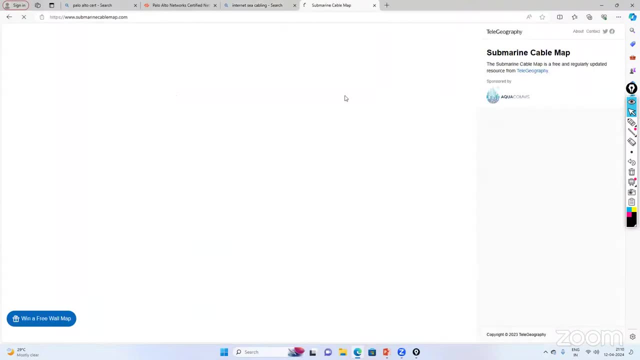 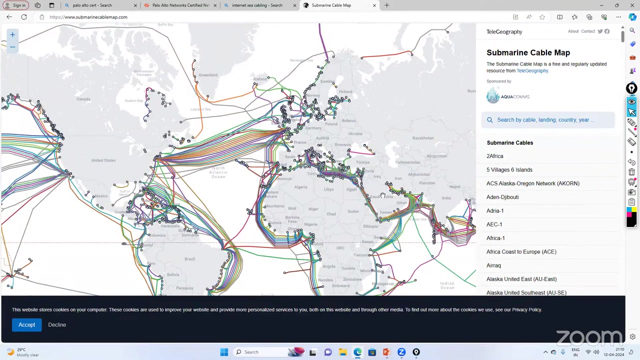 If I show you a map, then you will think that the internet is connected in this way. so if you see the C cabling of the internet, some people will also know about all this and some people will not. So if you go to this particular website- right, so you can see here which country from where their internet breakout is- 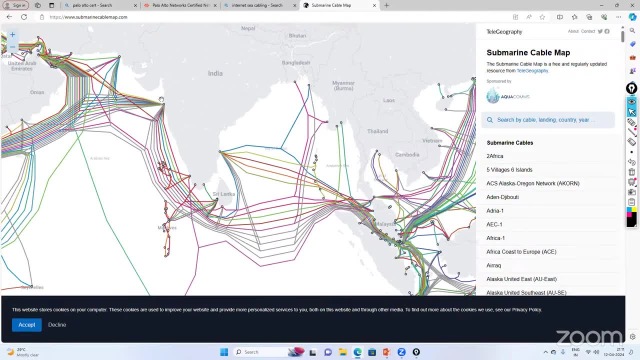 So if you look in India, then mostly our breakout is from Mumbai. Okay, if we connect with another country, right then they. So if we connect with another country, right then they. Our breakout is mostly from Mumbai. then there is also Chennai and there are two or three more locations here in Kochi. 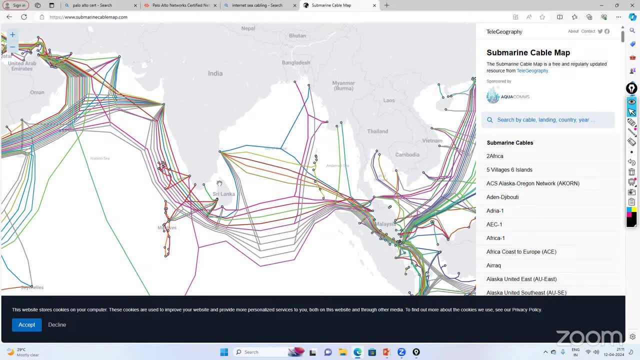 Okay, so this is our internet breakout location. Okay, if all these links are not working, then India is not connected to the internet. There are some services that run on satellite. okay, not all the services, so they can run, but this will not work. 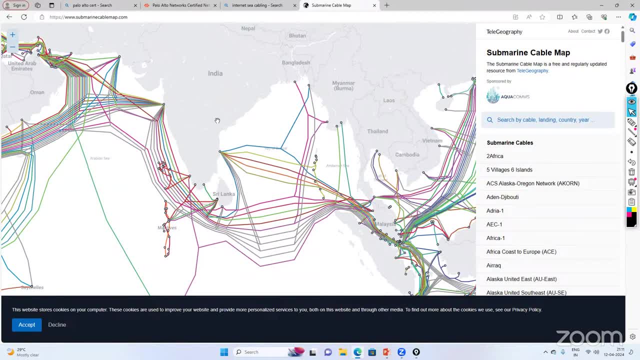 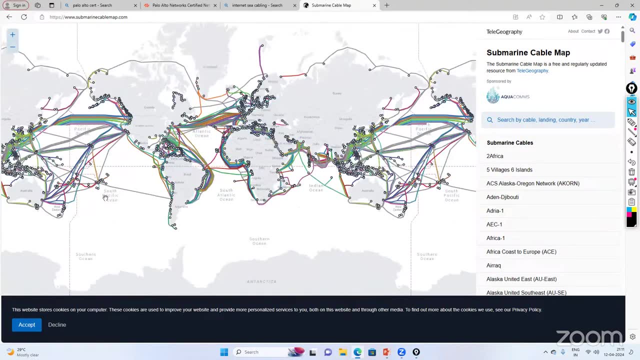 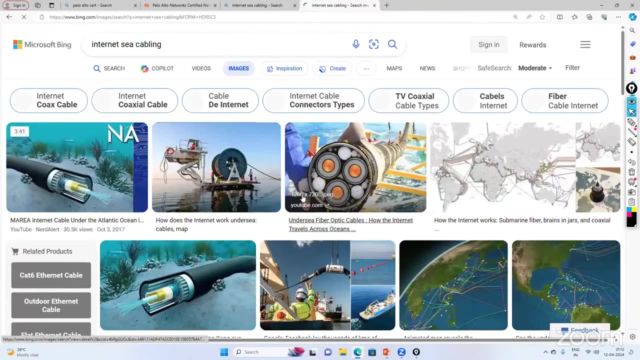 Okay, so in this way, if you want to see the map of the whole world, then you can see here and see how they are connected to each other. Okay, and this C cabling is something like this: If I go to the images and show you, then something looks like this: 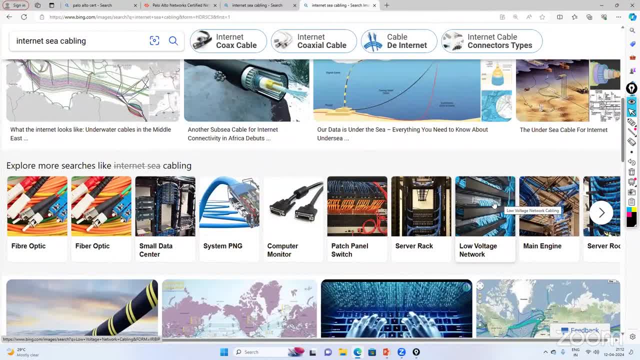 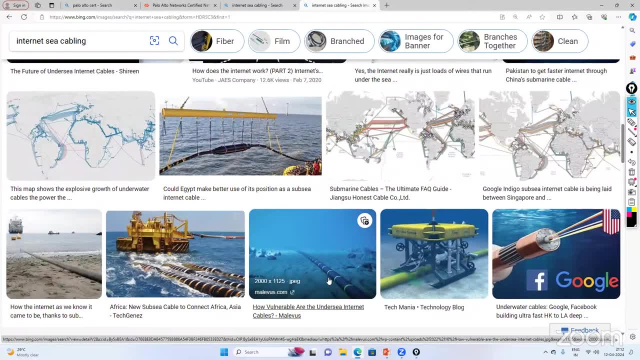 These cables are big, big, big cables and they also have some engineers who spread them And if there is a problem they also go inside and troubleshoot. Okay, if there is a problem in the cables, then at this level our internet is connected. 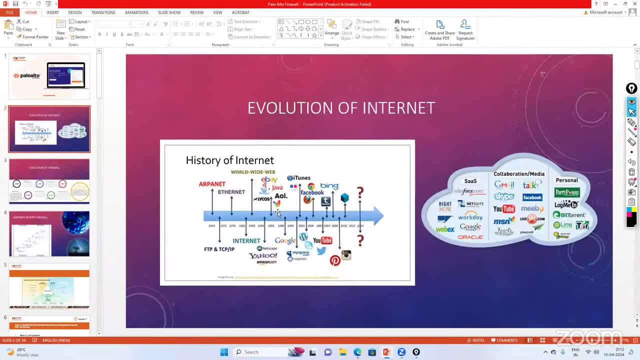 Now, how did this internet evolve so much? First of all, let's understand this. So when ARPANET? when the US defense, when they used ARPANET to talk to their army? After that, they gradually shared the file. 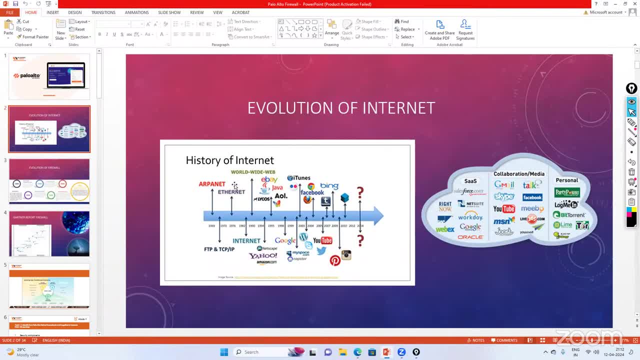 After that they gradually shared the file. After that they gradually shared the file. Then they started sharing the file- file transfer slowly. it changed to the internet. We started accessing the internet from different websites and the internet started evolving slowly. 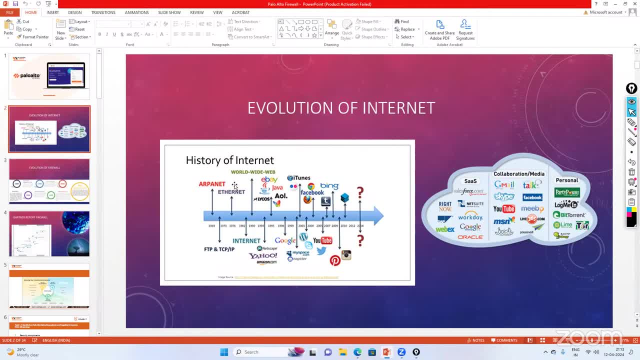 When there, for example, I made my website and hosted it on the internet. Now other users are coming, accessing, they are getting information. For example, there is a Gmail service so we are able to send mail. If one user is able to send mail to another user, then we start getting these advantages and we start using the internet. 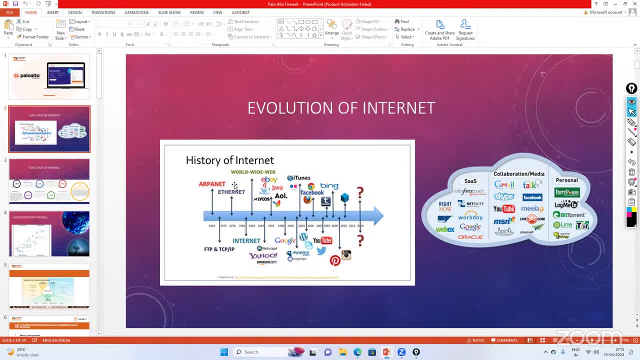 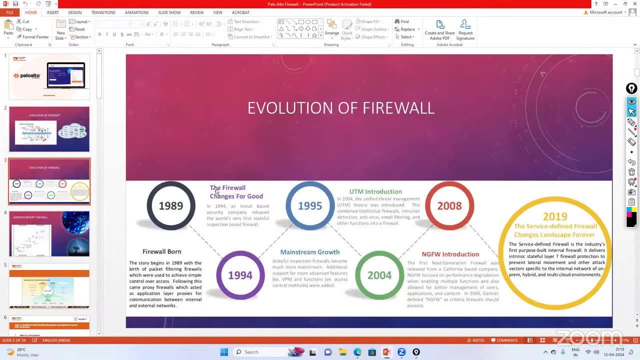 Where it is good, there will be some bad things also happen, right. So hackers started coming there, stole your information, started ruining things, So firewall was introduced in those cases so that they can protect that thing, So that when the user sends his information on the internet then he can securely transfer it from one place to another. 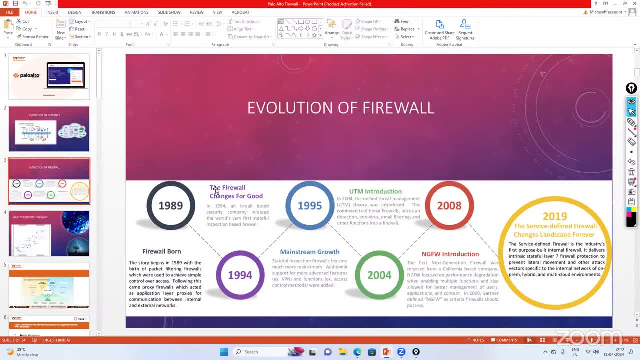 At the same time, when we work in a company like Apple, Pepsi, there are so many big companies like Tata, Infosys, There are so many companies. So if we want to protect their network, then when the traffic is coming from outside or from inside, then firewall is needed. in that case. 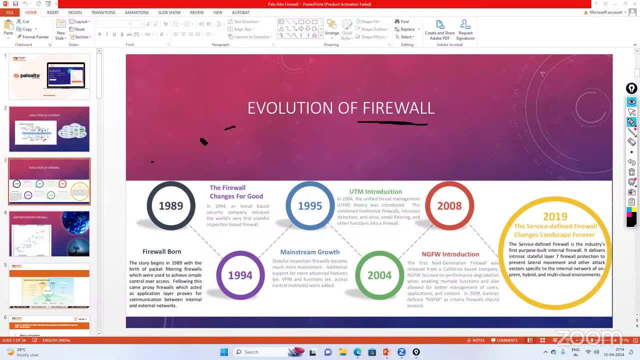 Whenever any external traffic comes to our organization from outside, then our firewall checks whether it is correct or not. How will it find out, When we give it some parameters, That here is the network? You have to check this IP address. You have to check this IP address. 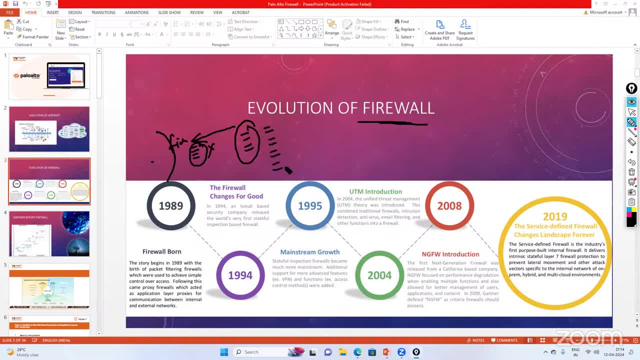 This port number or this application. So the way it evolved, the same way firewall also evolved. First firewall understood IP addresses, Then it understood port number. After that it also understood applications, Then it also understood all the applications in the application. So today the next generation firewall is the application that runs inside the application. 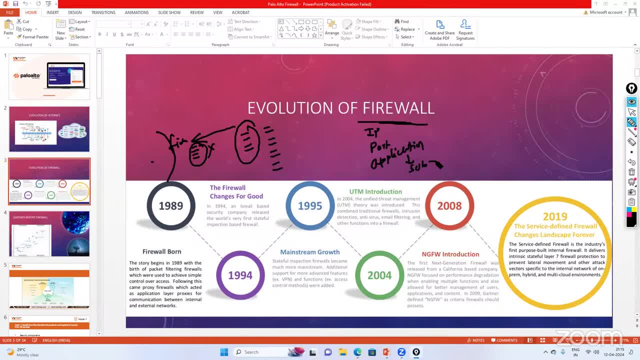 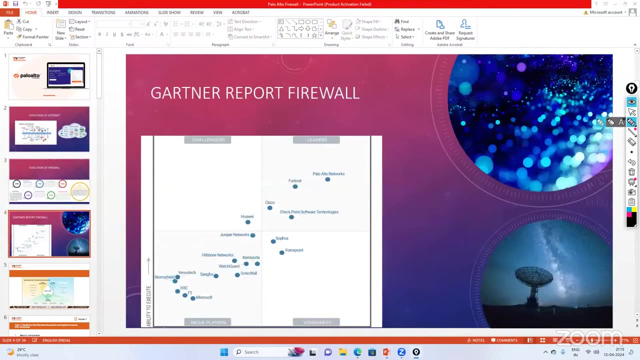 All the applications that are running, all the applications have also started to understand them Right Now. why are we focusing on firewall or Polo Alto? What is the reason to focus? So the reason is that Gartner is basically an independent organization. 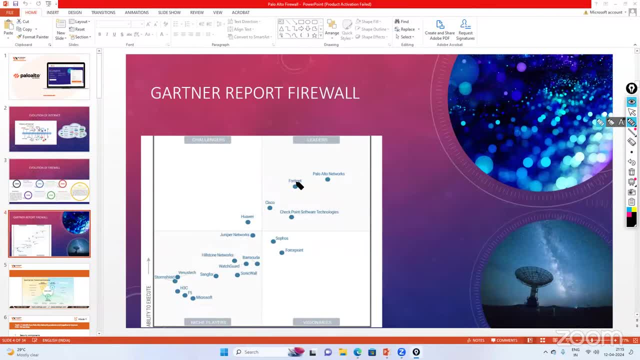 What reports does it release, Like what is the performance of any firewall, How is it, How is it not? How does it perform in any situation? So in that report the Polo Alto firewall basically comes to the leaders Right. So if it comes to the leaders it means this is the best firewall because it is doing. 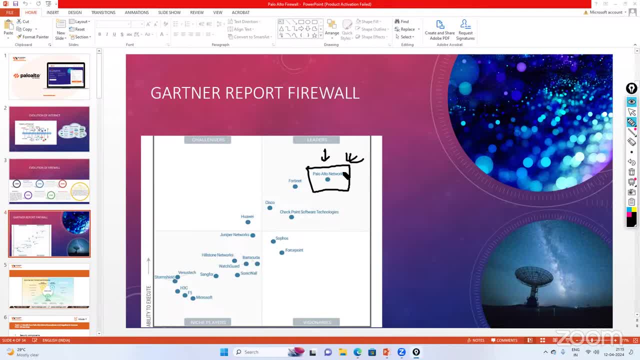 Excel in the performance test Right. So in the same way, if you look at the market of Polo Alto, then in every organization you will see Polo Alto. I am not telling that there will not be Fortinet, It will be there. 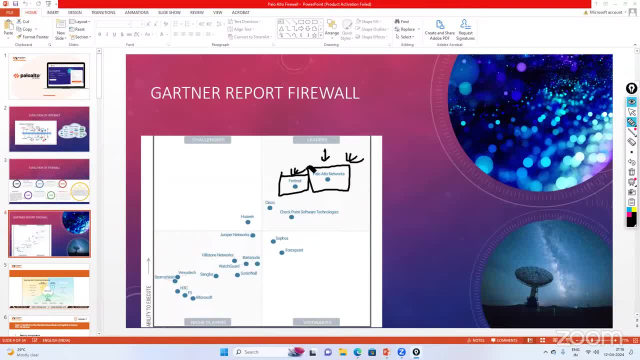 But Polo Alto's firewalls or customers are more. So if you know Polo Alto firewall, then you have more opportunity, because this deployment is in every and mostly most of the organization. So when it is in most of the organization, then you have more opportunity. 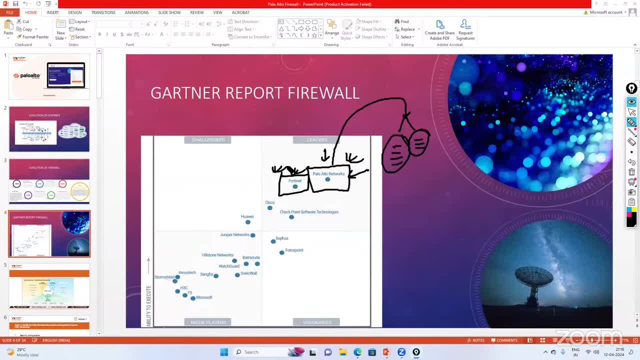 Right, I am not saying that you should not learn Fortinet. Fortinet is bad, Fortinet is good, Cisco is also good, Checkpoint is also good. They are very good as well in their places, whatever they does, Okay. 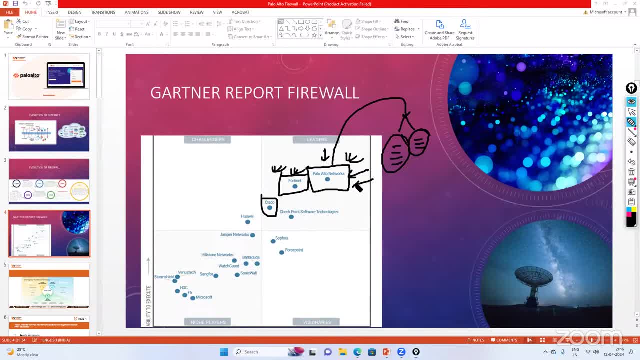 But as if you know the firewall, which is leader in the market, you can also understand Checkpoint as well. There is no problem Because the technology is similar, The way it configures, The way it works. little bit here and there You will be seeing in Fortinet or Polo Alto firewall or Checkpoint or Cisco. 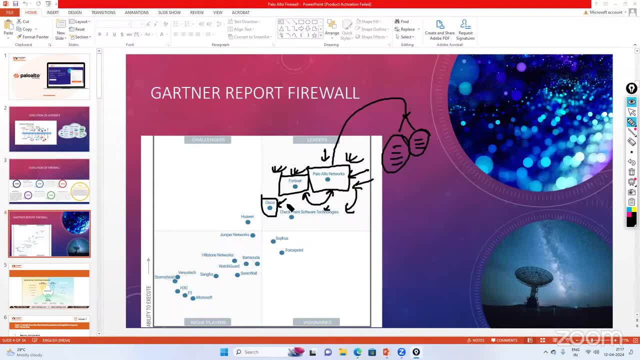 Okay, There will be a little difference, But it is the same Technology wise, like app ID works like this. It will work in a little different way. in Polo Alto, It will work in a little different way. There will be some configuration changes. 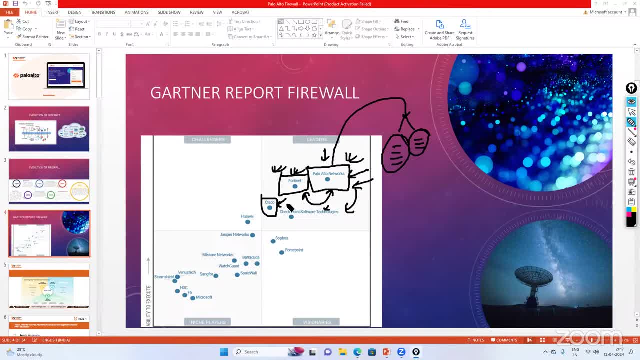 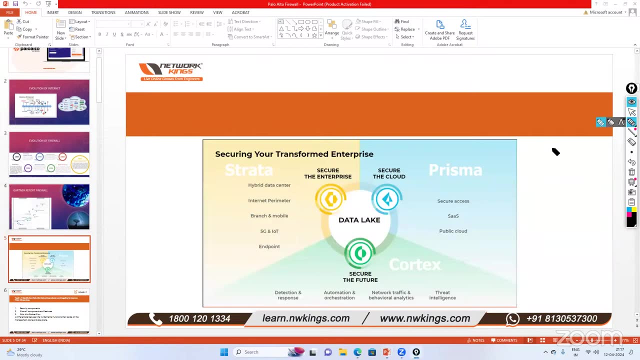 That's it, Okay. So if you are learning, then learn best firewall So that you can, So that you get more opportunity Right Now. Now let's talk a little bit about Polo Alto devices As a company. what are they doing? 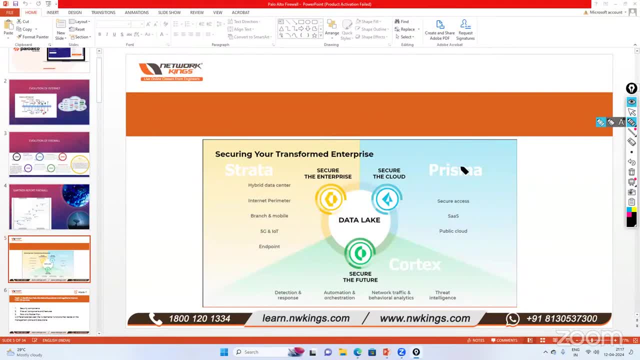 What are their portfolios? We will discuss the whole portfolio in a very good way, in a deep level, But right now we understand a little bit about them, about their portfolio, Okay. So first of all, let's talk about their portfolio. 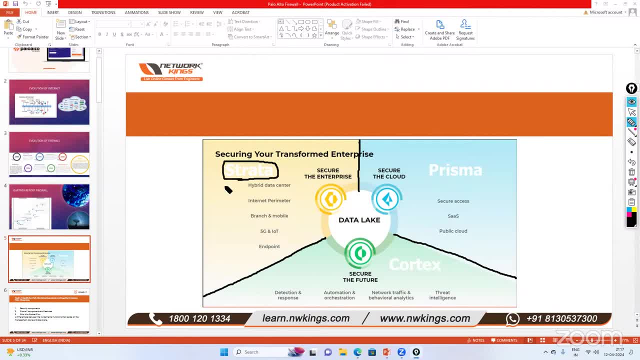 Okay, So Polo Alto has divided its product into three categories. Okay, One is Stata, one is Prisma and one is Cortex. So we will understand their target. What is their target? So what is the target of Stata? 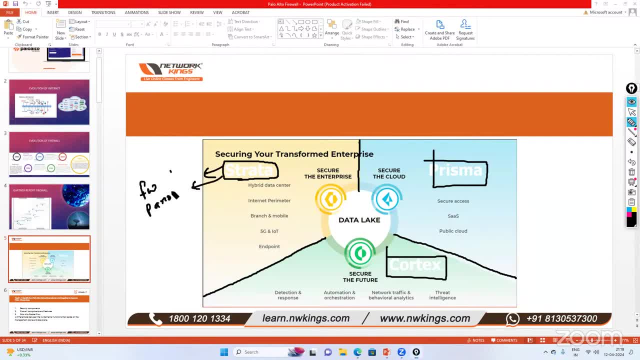 That this firewall is basically focused on Panorama. Now, this firewall I said is not just a physical firewall. There are virtual firewalls too, And there are different other types of firewall as well. Okay, In that we will cover which firewalls are used in internet firewalls and endpoints, and 5G and IoT. 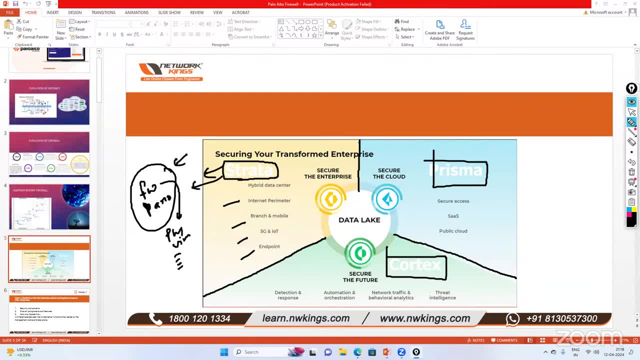 They have different models. We will discuss those, For right now, you understand, firewall and panorama are their main focus. Okay, Now what is Prisma Right now? Right now, we are not in a traditional data center. There are many companies and organizations that keep some parts in their premises and some parts in the cloud. 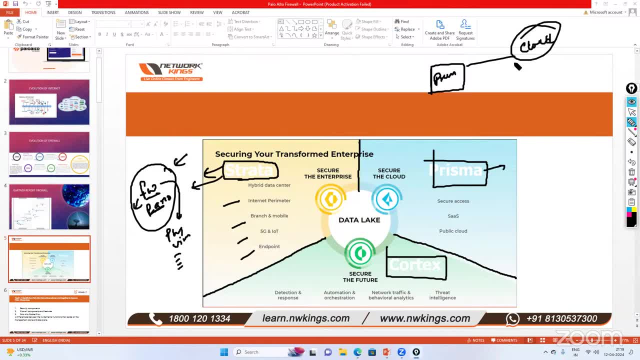 So what is it? It is a hybrid model. So, even if we have a cloud, Prisma will help you to secure your VMs, your compliance, Even they give you firewalls on rent, For example, we get a server on rent from AWS or from Azure or from many cloud providers. 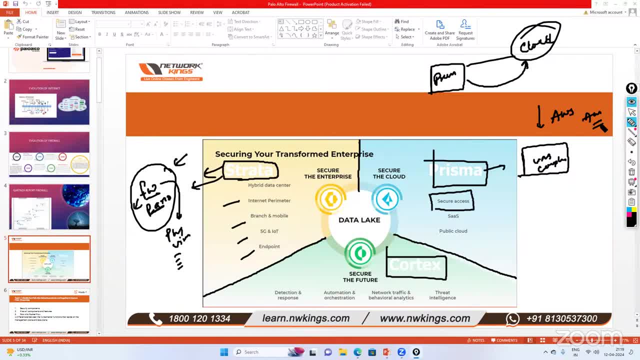 We get a server on rent. Similarly, we get a firewall on rent. So how will our connectivity be? For example, I am a user or I am a branch, So I will be directly connected to the internet And the firewall in the cloud. my traffic will go directly to it. 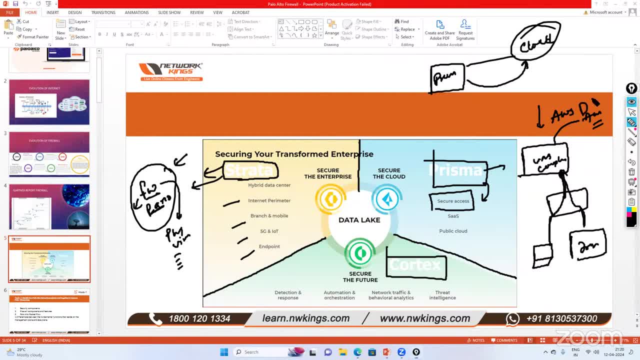 After that it will be filtered from there to my data center or to my headquarter or to the internet. Before that it will not go anywhere. So this is how it is configured: Directly traffic: If someone comes on the rent firewall and filters the firewall, his traffic will go out. 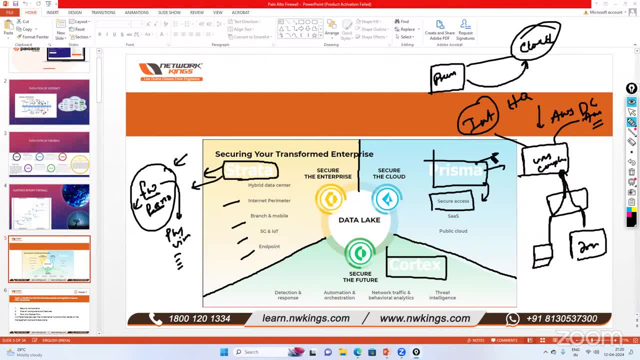 So in that way, we can also protect cloud devices from the cloud, And cloud firewall is also available. Now, what have we covered? We have covered physical, virtual devices and cloud. Now we will have a lot of behaviors there. 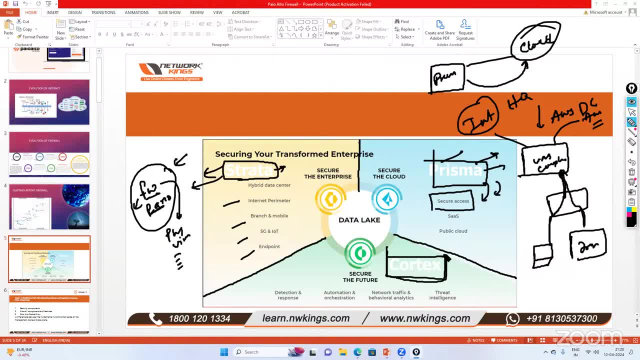 Like someone is attacking from outside in the physical environment, or someone is attacking in the cloud environment. So how will we protect that thing? There should be some mechanism to protect us, right? So there is detection and response. We have to analyze the behavior of the network. 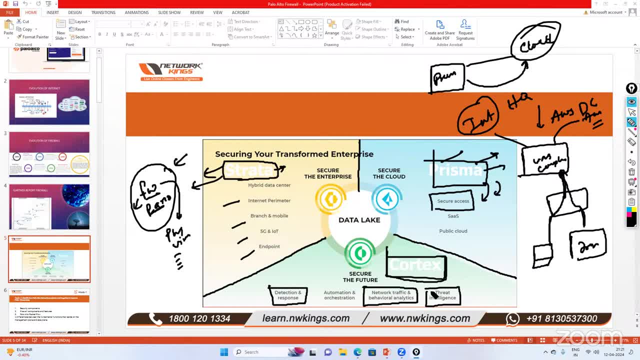 We have to build threat intelligence. So what will happen there? They will analyze and build that. this way, traffic should not come. this way traffic should come. So what intelligence will we build? When some response will come in that way, then what will be the traffic? 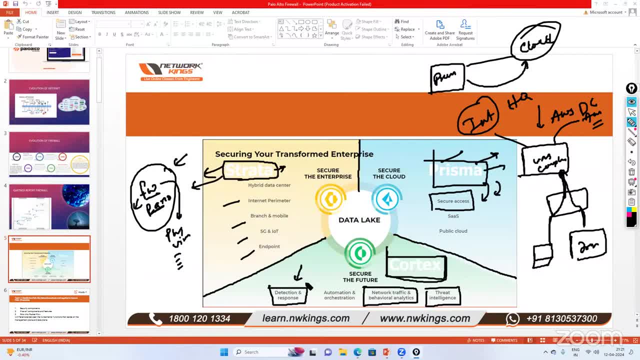 It will be denied, it will be blocked Right. And we also have automation. Polo Alto also has these services that it can automate things with the help of orchestration, So it can automate a lot of things for automation, Like if you want to implement a rule. 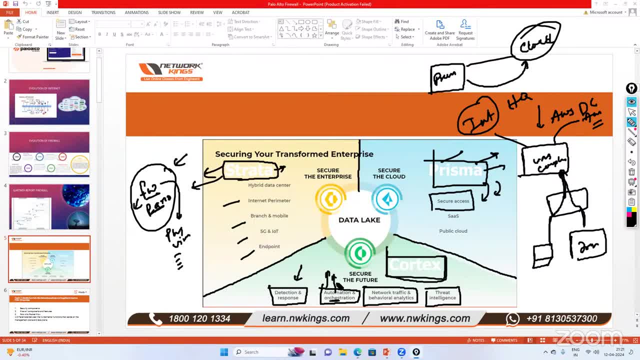 Or implement something in AD Or take a lot of things. This is very less. I am telling you. It can automate a lot of things with the help of orchestration Right And from your cloud, from your firewall and your threat intelligence network behavior. 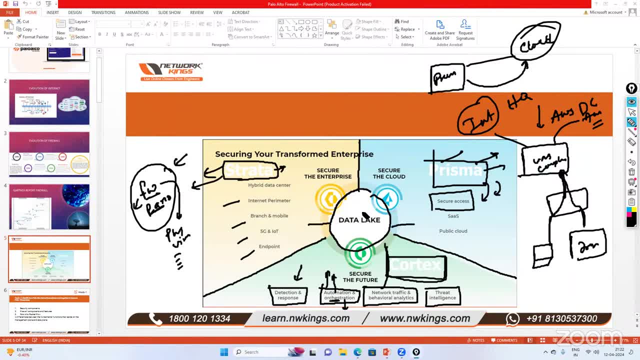 If you want to collect all the logs, then you can take the service of data lake from Polo Alto. You can store your all the logs over there. What is there in the device? You have a limit, But what is there in data lake? 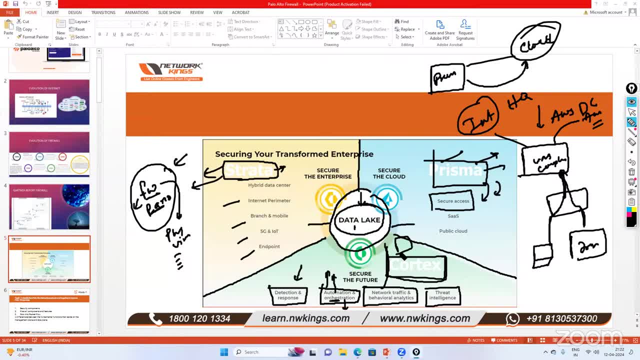 You can dump all the logs, all your previous logs. Let's say, for an example, that you want to store a year's logs, So you can get a storage from Polo Alto and you can store one year log over there. For, let's say, if you want to keep it for the next future use, then you can keep it like that. 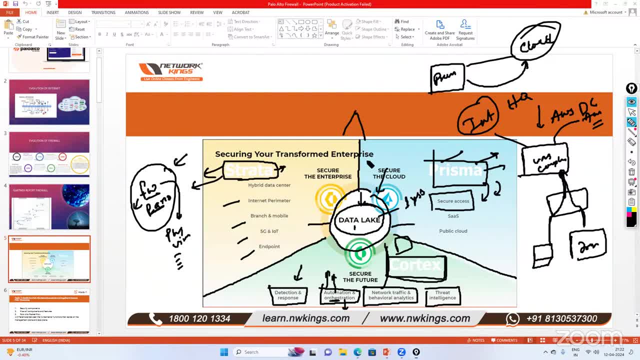 Right, So these are the models of their portfolio. We will study this in the next class in a more detailed way. Okay, Now we will see what we will cover in our courses, like in our series, And I will tell you how to cover it. 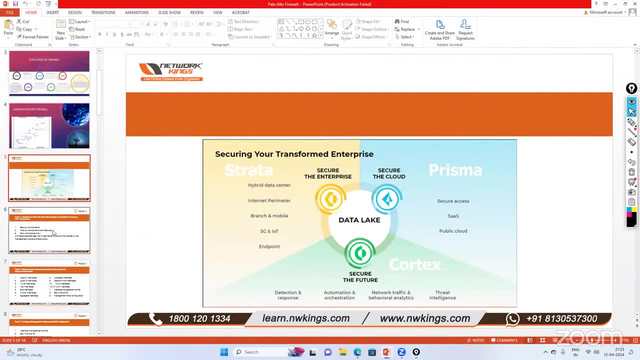 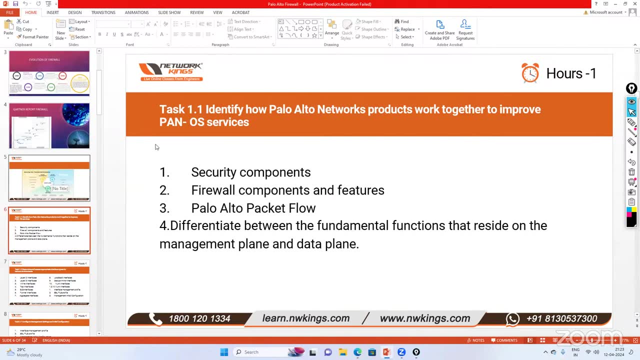 Okay, So if you have any questions then you can ask me, Or else I am good with this. Hello sir. Yes, Sir, what is the duration of the course? The duration of the course will be 45 days. 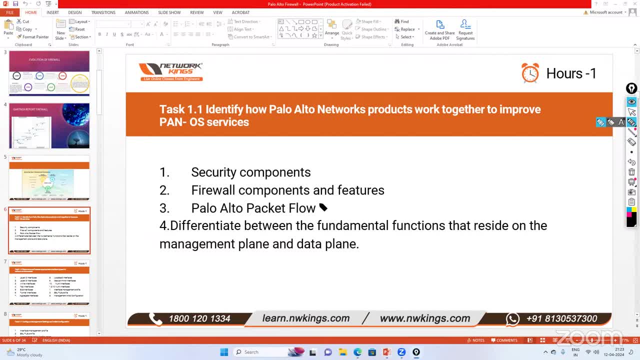 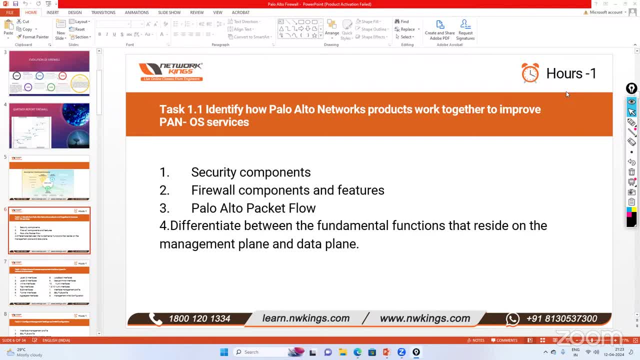 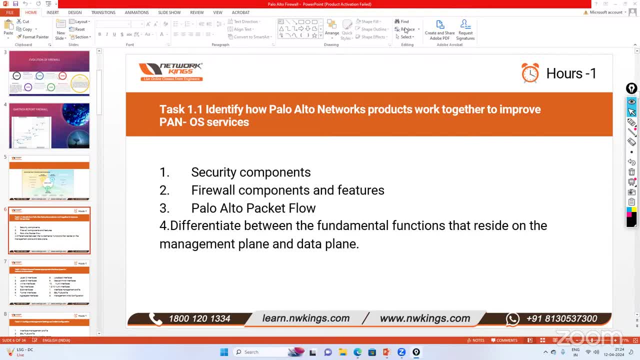 This is for the week days, Monday to Friday, So is there a weekend batch? Yes, Okay, Actually I enrolled for the weekends, So he gave me this. So is this the first lecture? Yes, this is the first one. 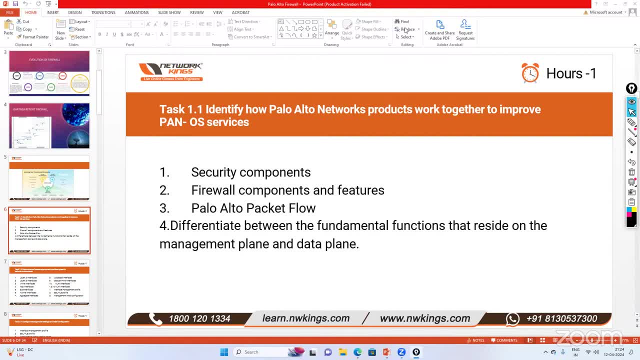 Okay, Okay, Yeah, first of all, Sir, when will the weekend bus start, sir? I'll have to ask this once Next time. The gore officer, sir. he must know. sir, OK, I'll inform him. 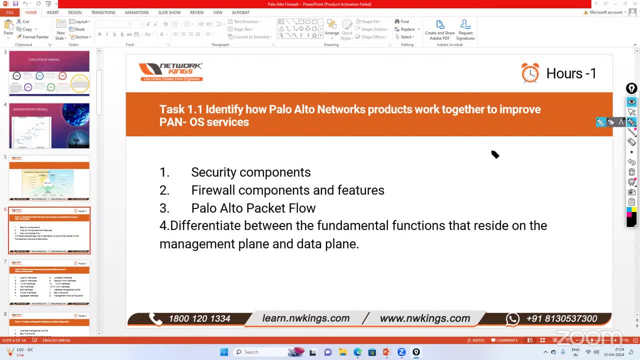 I'll talk to him. He has a schedule. OK, It will be yours, right, sir? the weekend bus- Weekend bus- will start next month. It won't happen this month. Next month's first year, second week. it will start like this: 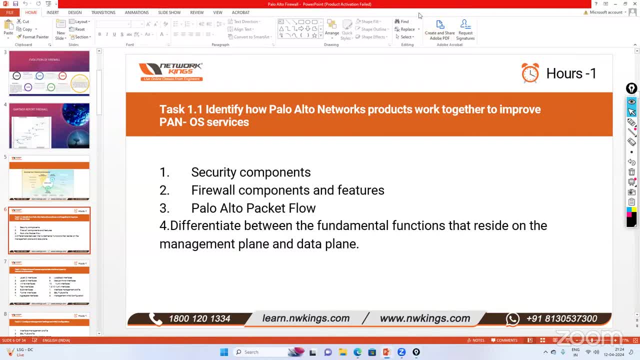 OK, OK, Will it be the same Sir? what will be the timing, sir, of the weekend: bus 10 to 1. Morning sir. Morning 10 to 1. OK, OK, OK, sir. 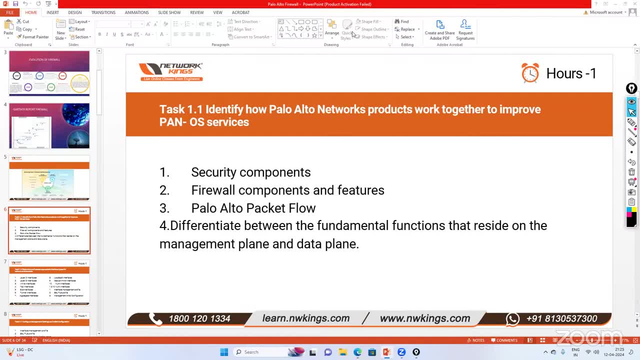 And it's 9 to 1,, right, That means weekdays No 8.30 to 10 o'clock. OK, OK, OK, All right, We will see. So, all right, guys. So yes, Everybody wants to take a picture. 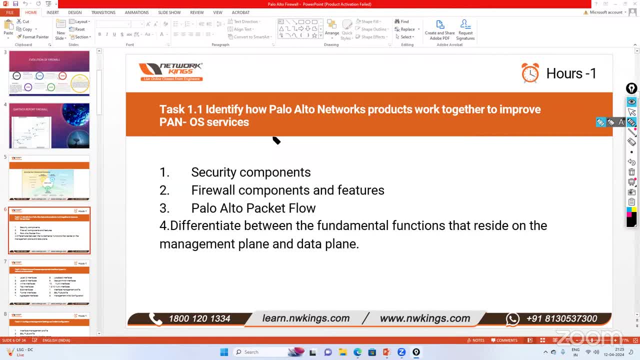 OK, got it. OK, Head, We are going to take an image. Does it look beautiful, guys? It was like a little prisoner on the lips, Just like this Question. share camera. Done udge research in preanger is of this bag, friend. 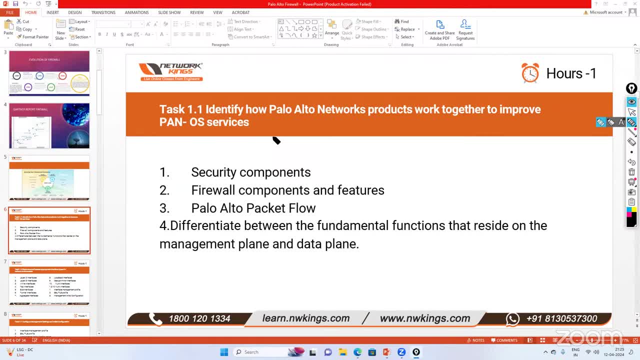 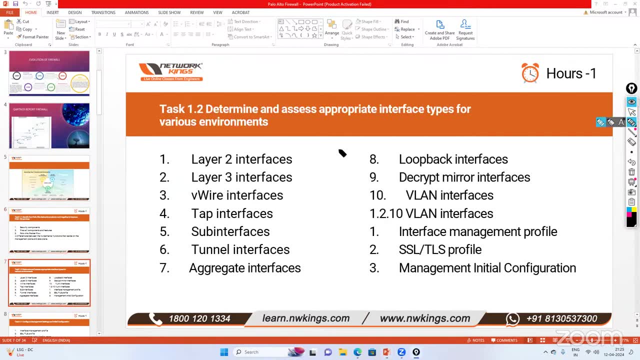 including the engagement plan. So at these are. so we will go The driver. After that we will go to its interfaces, because Polo Alto Firewall is so flexible that it can adopt any environment Where I don't want to change the IP address. I want to change the IP address. 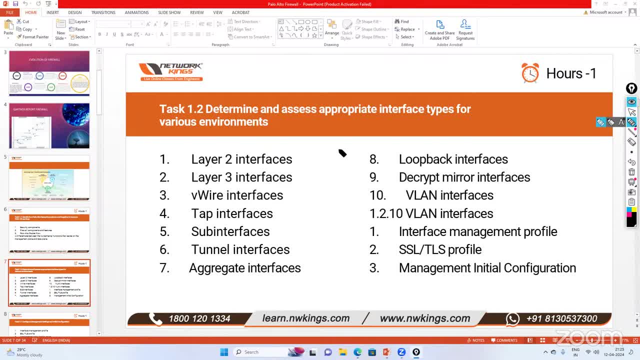 I want to run BGP in it, I want to configure VLAN. it is flexible for all things, So we will read about it, that in which scenarios, which types of interfaces can be implemented- Layer 2,, Layer 3,, VWire- then Tap Interface, Sub Interfaces. 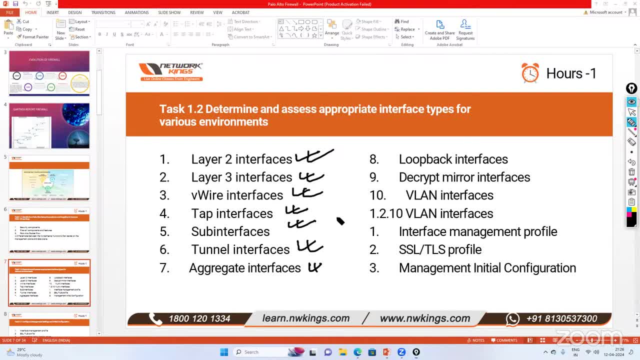 Tunnel Interfaces for VPN tunnels, Aggregate. so if you combine two interfaces, if you bundle, then Aggregate Interface, then Loopback Interface, Logical Interface, then Decryption, Mirror Interface, then VLAN Interface. We are going to cover all these interfaces in a very detailed way. 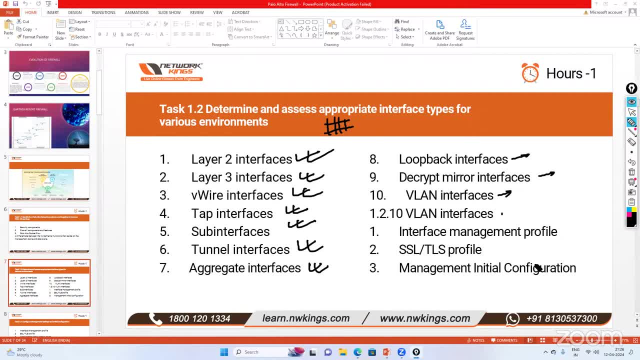 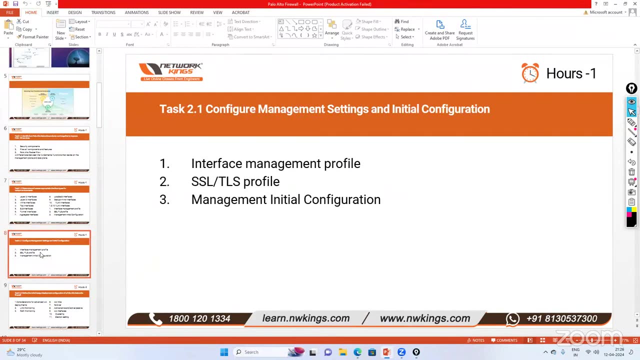 We will also do its practical. we will see how it is being configured. all this After that, when we come to the next topic: how do we access the device? Like which protocols should we allow? What should be the TLS and SSL profile? 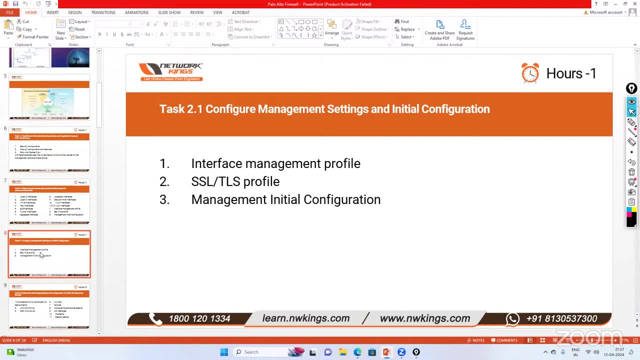 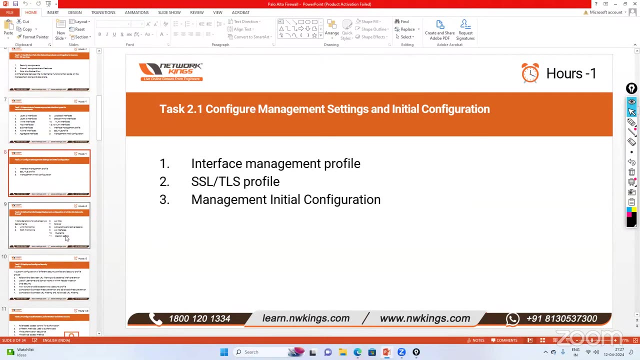 When we first log in to the device, which things should be configured first, Like DNS information, NTP information and some other information sources that we should first implement, right? So we will see all those things After that when we design the firewall. 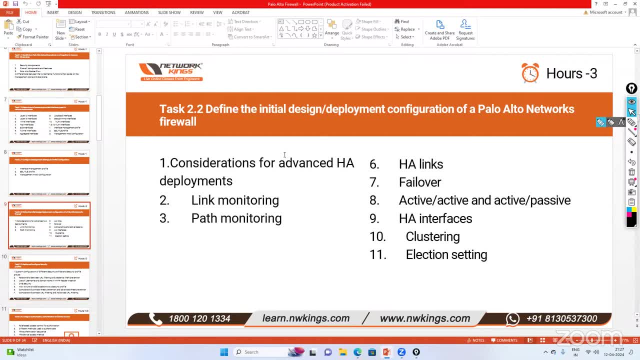 whether to implement HA in it or not or to implement standalone. when we implement HA, what should we monitor? Should we monitor the link? Should we monitor the path? Should we not do this? Or which device should we keep active? Which device should we keep on standby? 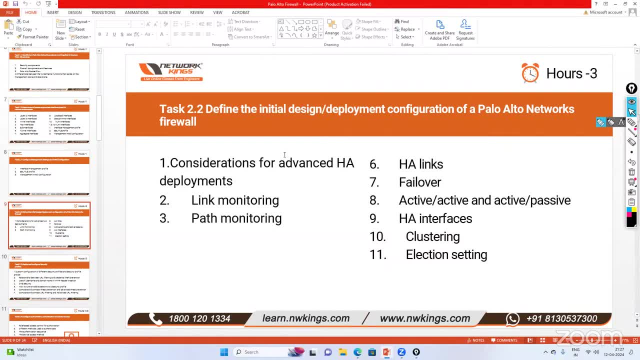 Or what kind of election process. So we have the control that whatever we want, we can do it for ourselves. right That if I want Palo Alto to want to be active, we will make it active If we want to make the second one on standby. 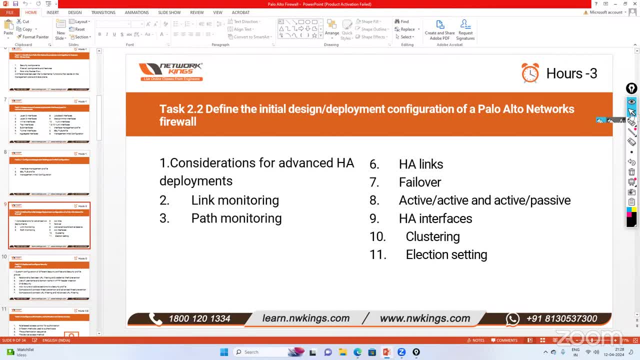 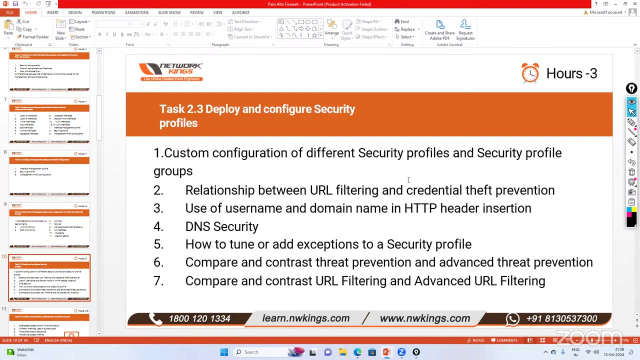 we can make it on standby. Okay, So this is how we can do it. So we will see all those things that, when we design which HA is needed or not, we will see all those things. After that comes security profile configuration. 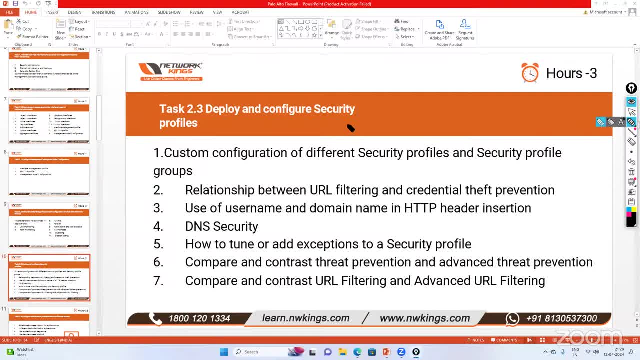 A lot of things come in the security profile, like content filtering- if I tell you then, URL filtering, your anti-virus, your anti-malware, file blocking. there are a lot of things that come in it. Okay, When traffic goes out of Palo Alto. 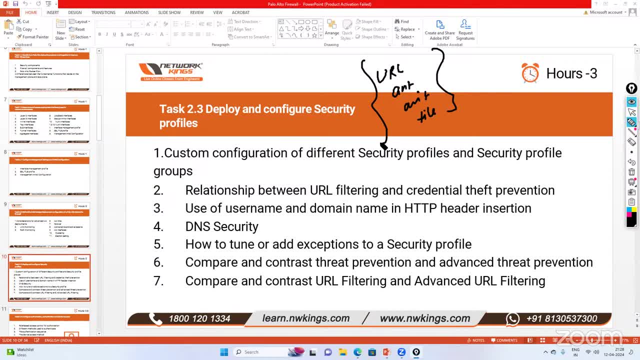 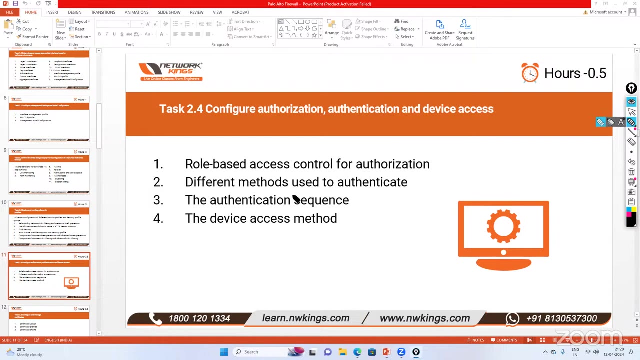 then which things should be checked? We check all those things from the security profile, Okay. And in URL filtering, what is advanced URL filtering Then? how do we put exceptions in the security profile? We will see all those things, Okay, When we log in to the device. 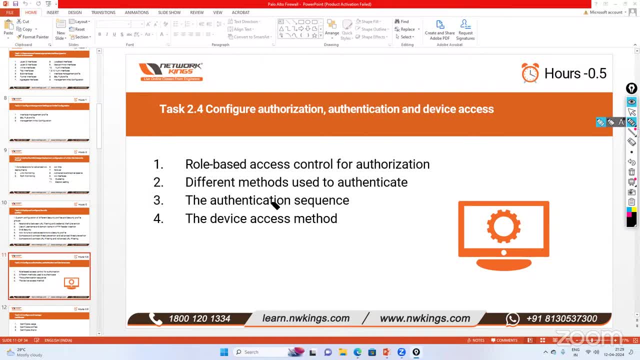 okay, then what access should we get Now? for example, if you are an L2 engineer, if you are an L1 engineer, L3 engineer, then they have some responsibilities, Right, The L3 engineer will be the last stage of troubleshooting. 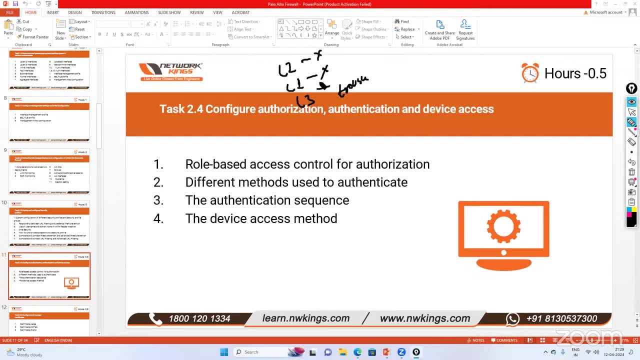 If L2 can't do it, L2 can't do it, L1 can't do it. Okay, So L3 will have more access to the device, L1 will have less, L2 will have more than that, Right. 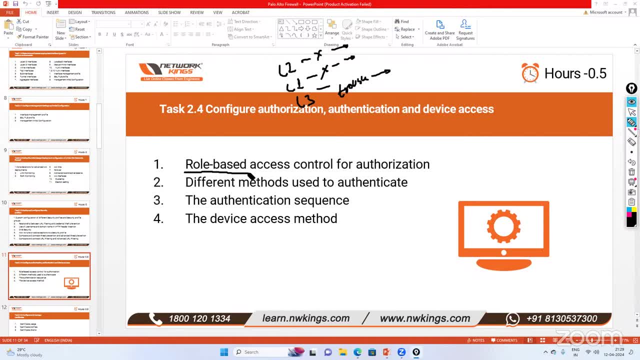 So we can define that role, that when a user will log in to the device, what access should he get, What authorization should he get? Okay, And how should it be authenticated? We can use radius for authentication. We can create a local user for authentication. 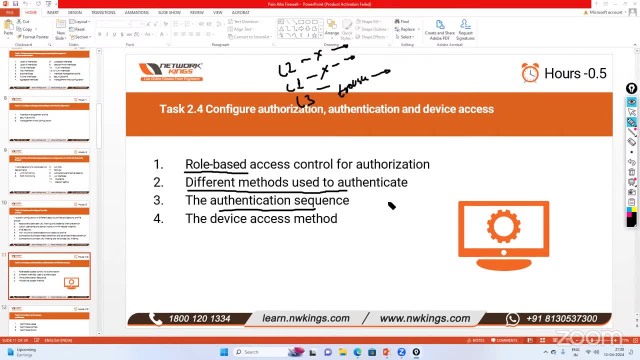 Right, And we can also tell the sequence That first of all, there should be radius authentication. If it fails there, then there should be TACACS. If it fails there, it should be local. So in this way we can define the sequence. 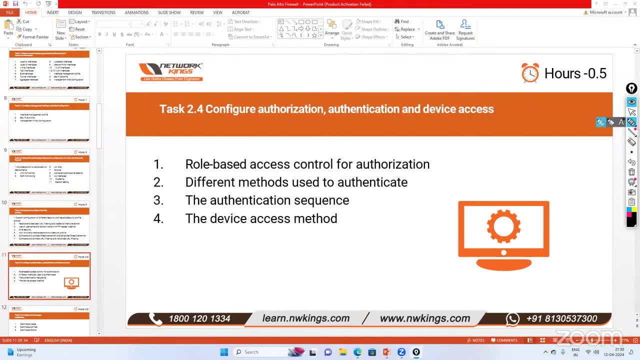 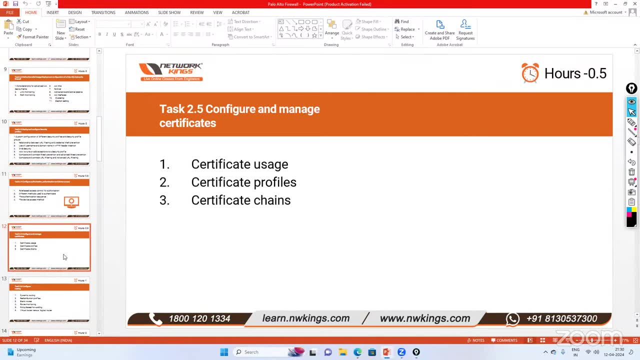 Okay, And in this way we can control the user Right. After that comes the most important certificate. Certificate means your public key infra In public key infra, how the certificate basically works. what is root CA? what is client certificate? 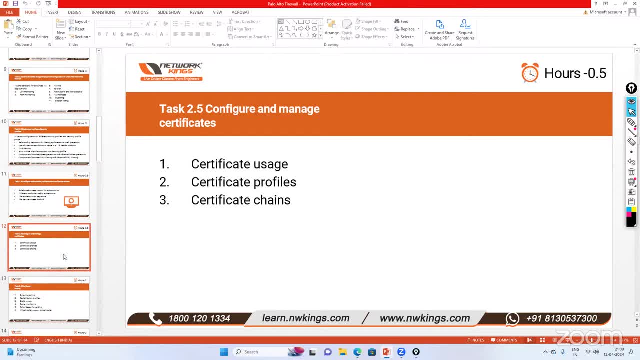 all these things we are going to talk about here. How does it work? Because there is an important thing in this, which is SSL decryption. We will learn how SSL decryption works, In that the certificate plays a very big role, So we will understand it very well. 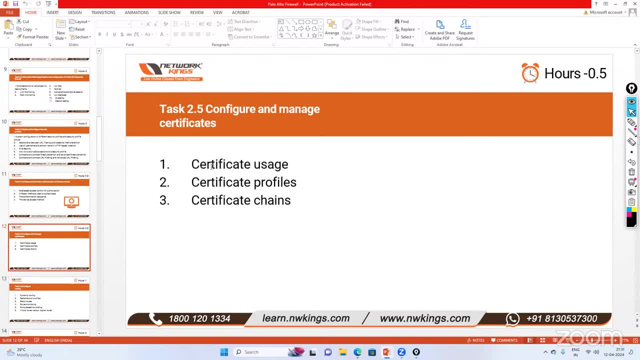 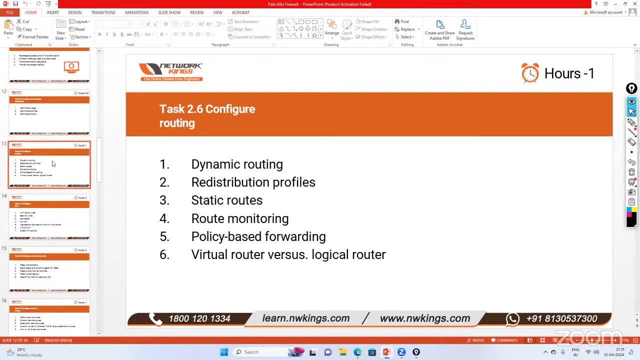 What is the usage of certificate change or certificate profile? We will understand all those things. After that, as in Palo Alto Firewall, we can cover and configure dynamic routing, static routing, redistribution, all the routing things. Okay, We will see all those things too. 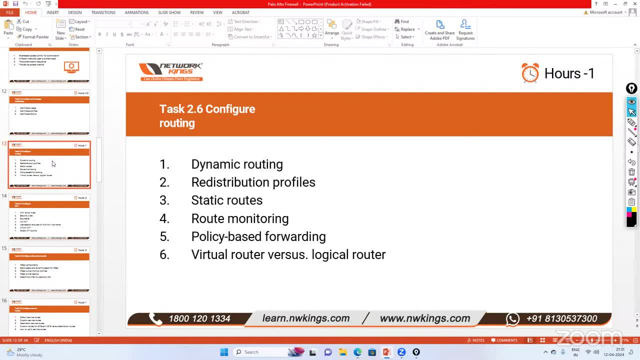 There is a new thing in our Palo Alto, which is virtual routers. We can make different routing tables In one firewall. we can make 3-4 routing tables, Okay. So we will do that too in this way, And one is forward. 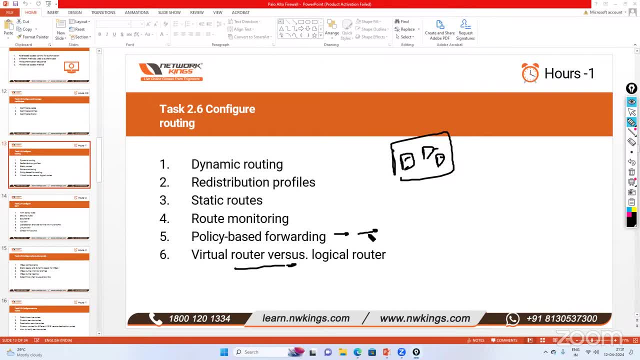 This will be available in all devices or in firewalls: Policy based forwarding. So if we have two ISPs, Okay, If we want that, my first ISP will take all the traffic from 10.0.0.0 slash 24.. 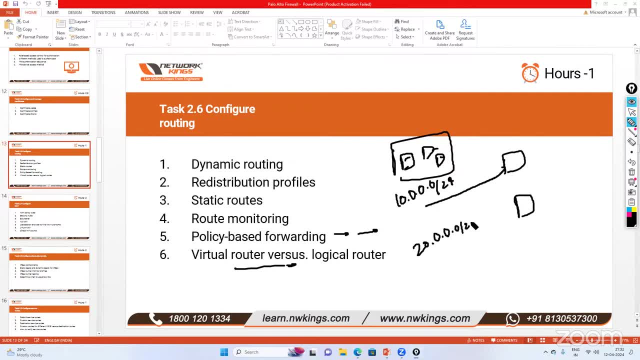 If somebody is coming from 10.0.0.0. slash 24, he should go from ISP 2.. So we can configure this way, with policy based routing, That we can force the traffic that you go from ISP 1,. 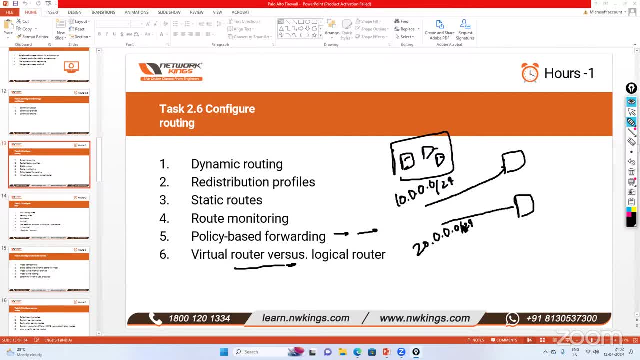 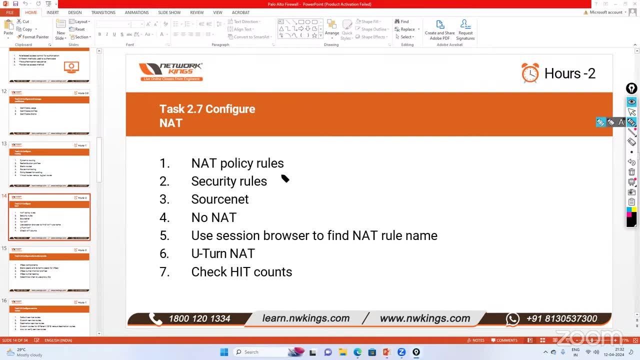 you go from ISP 2. So we can do policy based routing, which we are going to learn. Okay, NAT: NAT is a very important topic because every organization needs NAT, Where we do address network address translation, Even if you are connected. to Wi-Fi right now, then you are NAT. Even all ISPs do NAT. They NAT your traffic and send it to the internet. There are not so many public IPs. Everyone cannot get public IP address, Okay. So how many types of NAT are there? 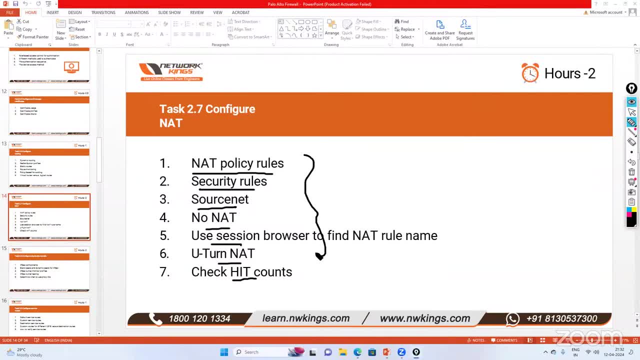 How do they work? What are the troubleshooting steps? I will be covering everything. Okay, So everything will be covered. What are the possibilities in follow-alto? destination NAT, static NAT, everything Okay. After this comes site-to-site VPN. 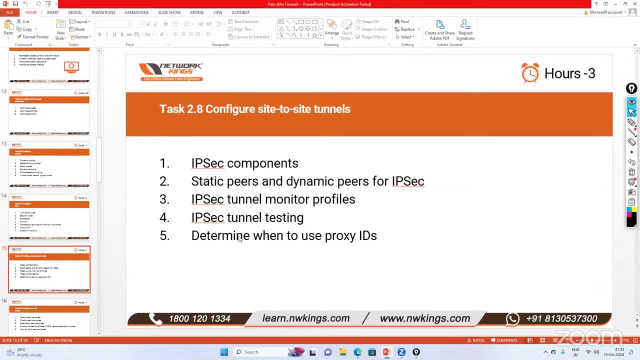 Site-to-site VPN means that if one branch wants to be connected privately with another branch, for example, we have follow-alto 1, follow-alto 2, this is our private network. this is our private network If they want to talk. 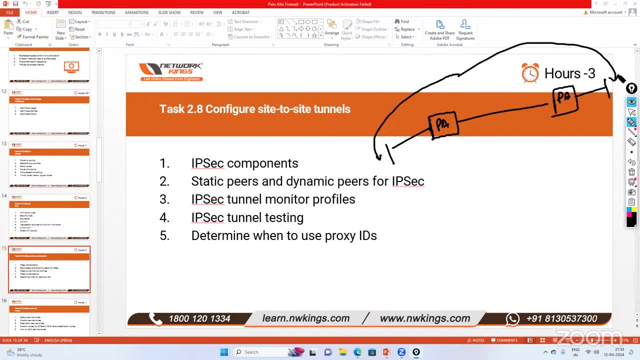 through the internet, through these two private networks, then how will they talk? Because here also there is a private IP address. here also there is a private IP address. So how will they talk? Because on the internet private IP address is not routable. 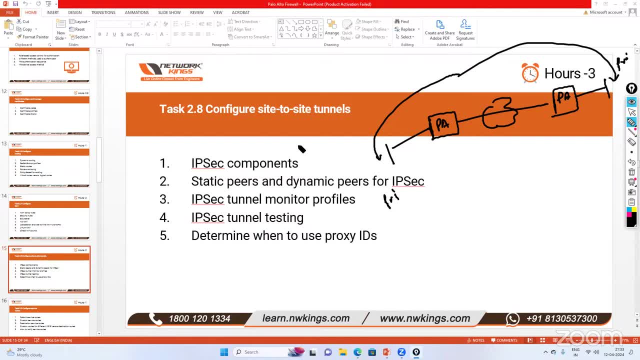 Through the tunnel? it is possible, And how will they do it in follow-alto? we are going to see, And I will also tell you a trick- that if you do site-to-site VPN from follow-alto on any other device, I will tell you that trick. 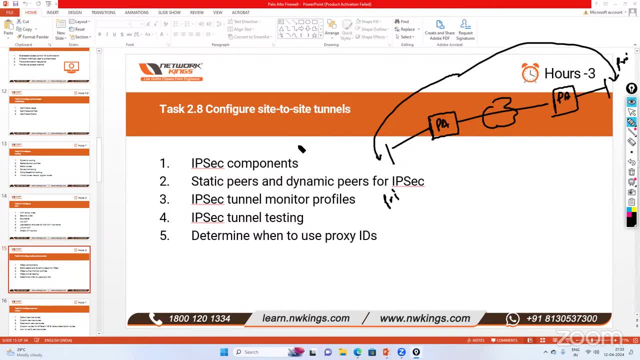 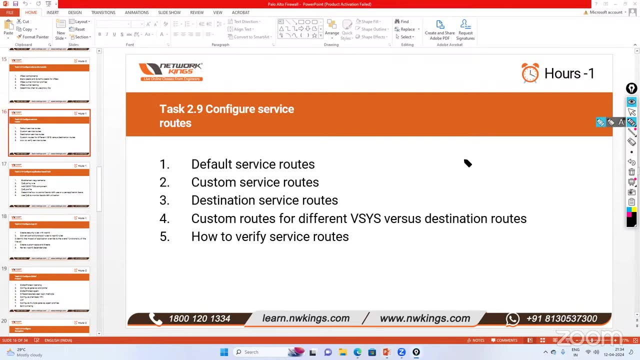 that. how are the possibilities Like follow-alto 148, or Cisco or other devices, then that is also possible. After that comes service route. Service route is a very easy topic. For example, this is our follow-alto. 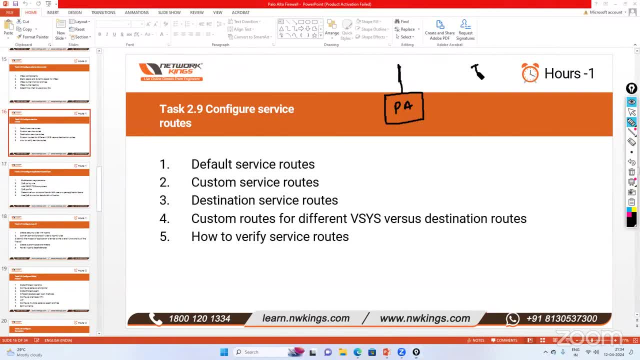 So by default all my traffic- like if I want to configure TACACS, communicate TACACS, TACACS plus, or I want to talk to DNA, or I want to talk to NTP, then by default all my traffic will be going through. 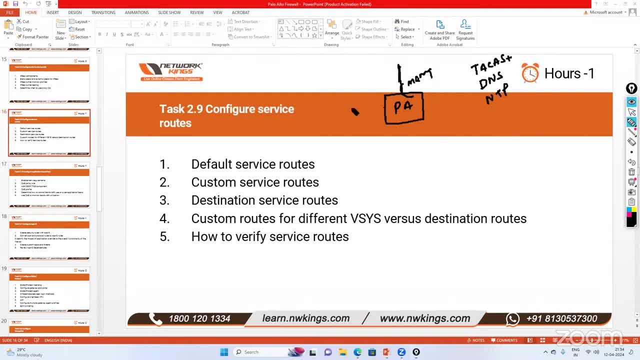 management interface, But my TACACS, let's say my TACACS- is reachable via 1 slash 1.. If my DNS is reachable via 1 slash 2,. if my NTP is reachable via 1 slash 3,. 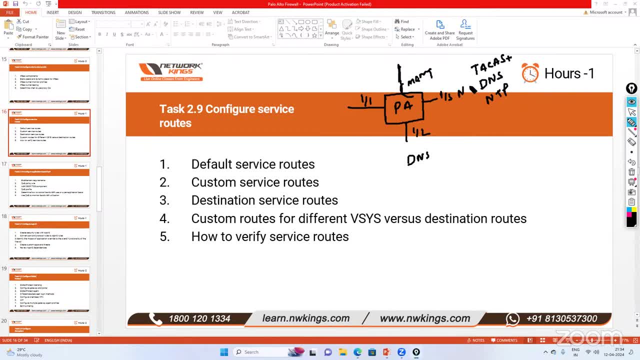 so here is our DNS, here is our NTP and here is our TACACS. Okay, So in this case what will happen is if all the traffic will be going through management, then it is not possible to reach. 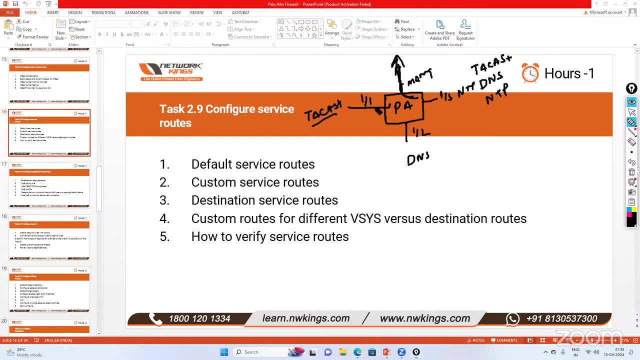 So we will go to TACACS and say that this is reachable via 1 slash 1.. This DNS is reachable, So we will basically tell the traffic of control plane that you can reach this service through this interface. Okay, If you are not able to understand what it is, 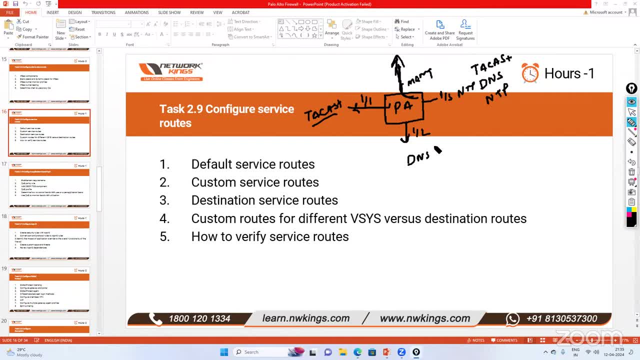 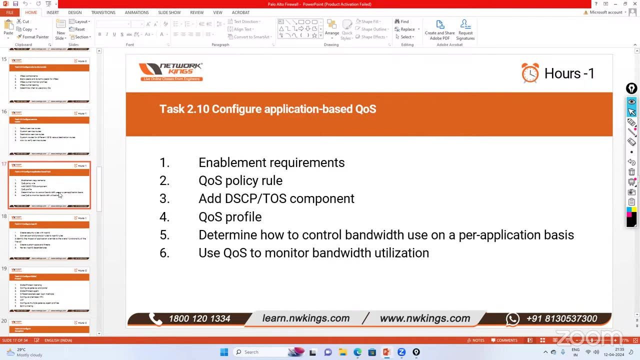 I will tell you, I will cover it in detail, So don't worry about it. If you are not able to understand, then you can understand. Do it Okay? Then QSS. So if, let's say, you want to give quality of service, 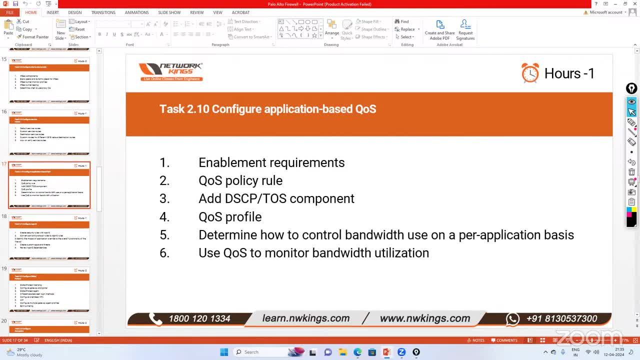 to a specific application, then you can give it easily. Okay, Let's say you want to give WebEx, If you want to give QSS service to WebEx, because what happens is that this is a collaboration, this is an application. 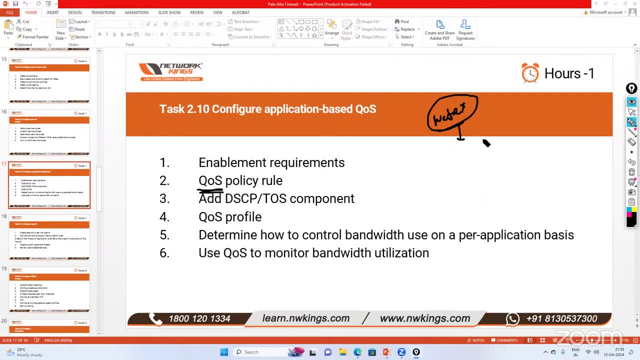 and in this urgency, like quality of service is needed because this is a video call, like in video conferencing, So in that case QSS is necessary. So if I want, then I can apply QSS policy only for WebEx. 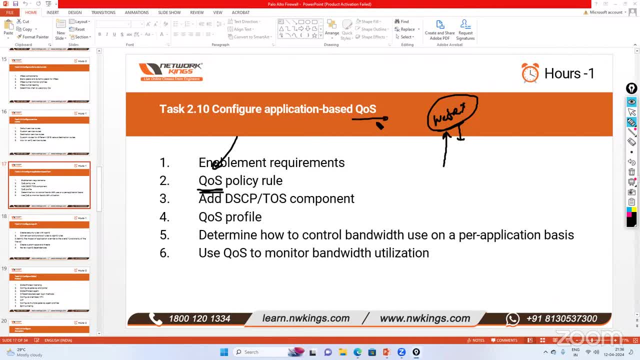 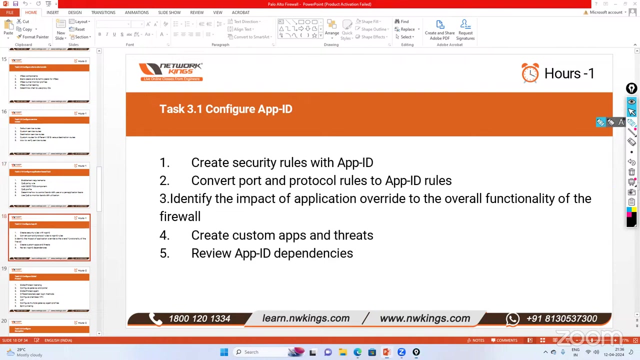 And that too, only for that particular application. We don't need that. we have to involve other applications also. No need, Okay, It can be on application basis. Okay, After that comes application ID. Application ID is so strong and works in such a good way. 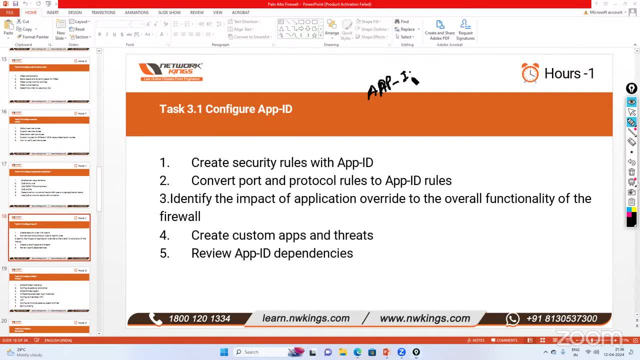 application ID that if you like running Facebook- there are many other applications in Facebook like charts or games- then they also need to be blocked, So you can block it And there is a process to block it or to understand it. 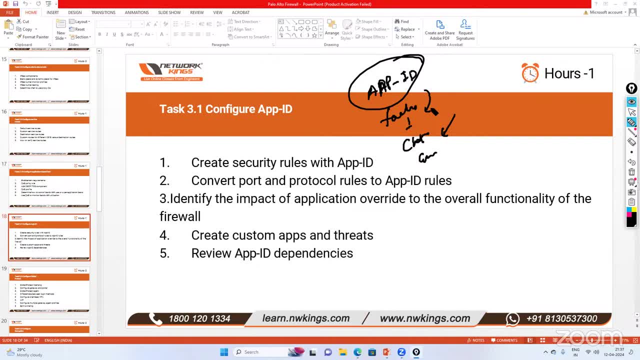 to understand its concept. I will cover that in a very detailed way So you will understand how the traffic is going. first the followers are understanding it, then it is blocking it, how it is blocking it. I will cover all those things. 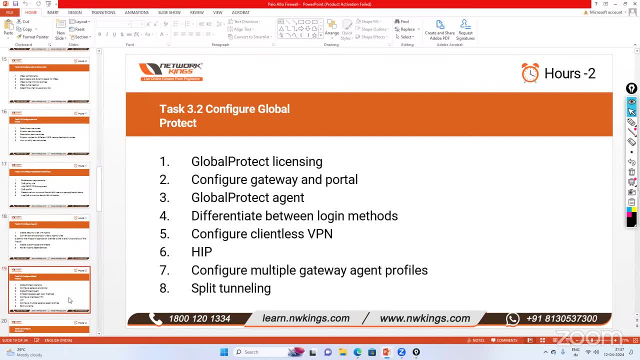 Okay, Then comes Global Protect. So if you are working in any organization, then you must have heard the name of Cisco AnyConnect Or Forti Client Global Protect in Palo Alto. Okay, So what is this? This? if you are sitting at home, 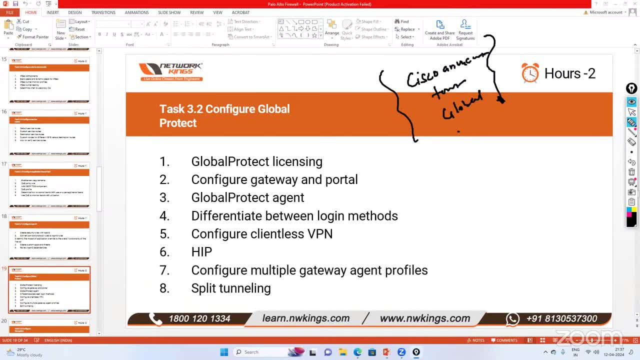 and you want to do your office by sitting at home. so what is this? This is a solution so that remote users can connect to your organization and can do your work if you are not available in the office, If you are traveling somewhere or if you are working from home. 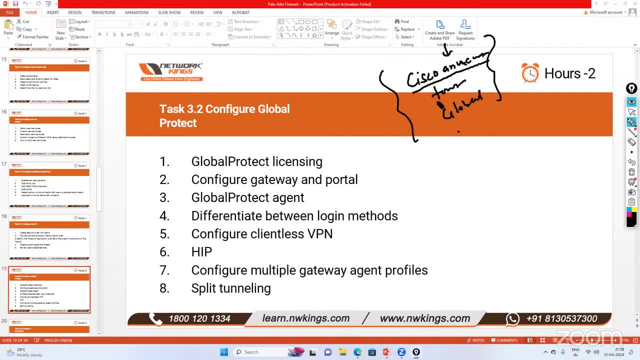 these are the solutions. So the way Cisco AnyConnect works or Forti Client works, the Global Protect also works the same way. there is no difference. There are few things which is changed in Global Protect, but the concept remains the same. 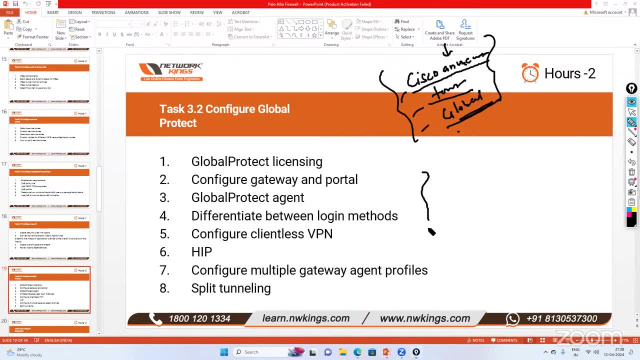 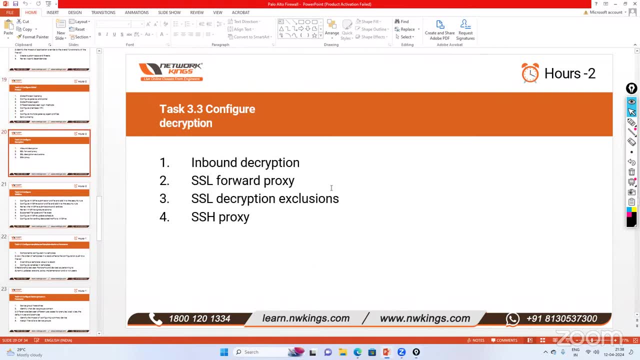 for remote users, Okay, Which we are going to cover it. Then we have configuration decryption. So if, as I told you, that one server or, for example, there is one user and he connects to one server, okay, That traffic is HTTPS traffic. 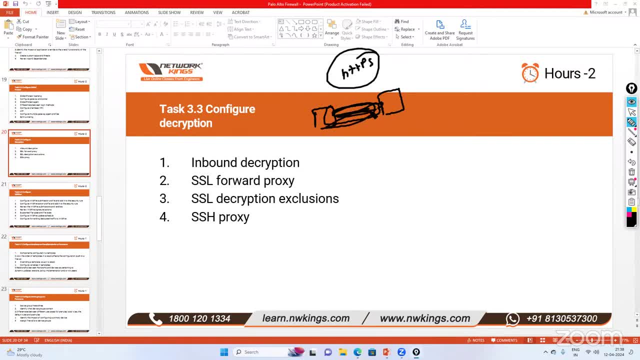 So what will happen? It will create a tunnel and will send traffic from the tunnel. Now, in the middle, Paul Aalto is standing and he doesn't know what the traffic is sending: from the user side to the server side or server side to the user side. 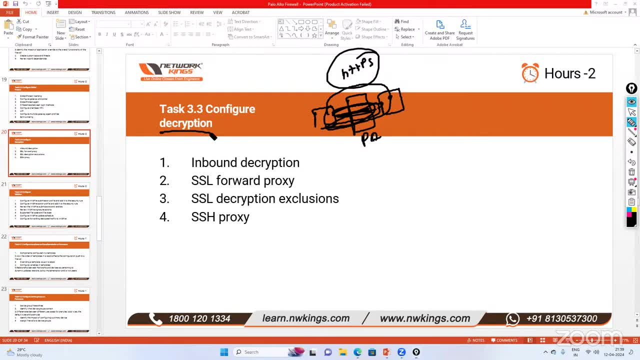 Right. So in that case, decryption plays a very important role so that he can decrypt and see what the user is sending to the server and what the server is sending to the user In the middle, if there is any malware or if there is any attack. 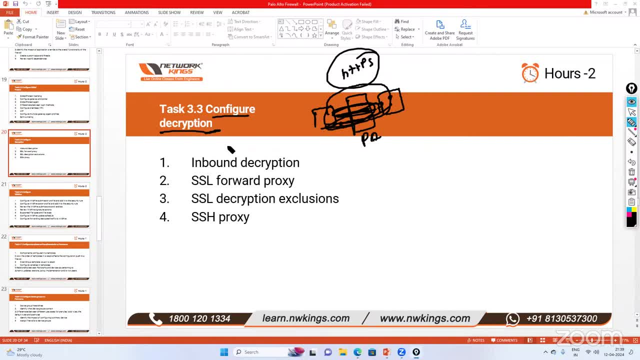 So in that case decryption is needed. If we go to an unknown or such a website which is not popular and we don't have any idea about it at that time decryption is very useful Because if it injects malware through the tunnel, 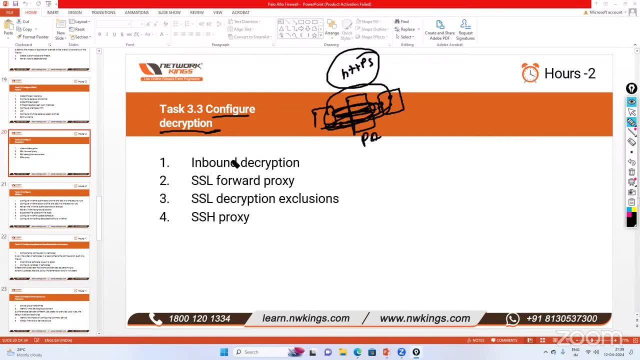 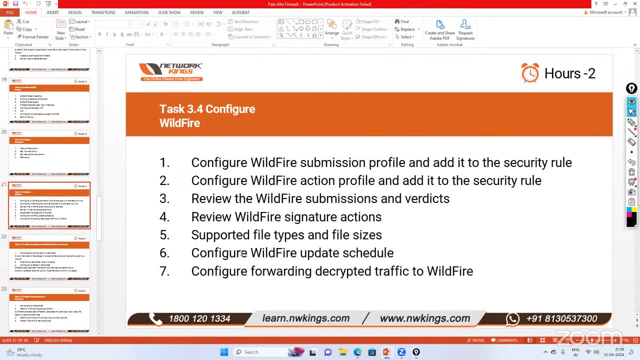 Paul Aalto will never get to know that something is coming in between. Okay, So decryption is very major. After that, you need to do one thing. It is called wild fire. What does wildfire do When you download or upload a file? 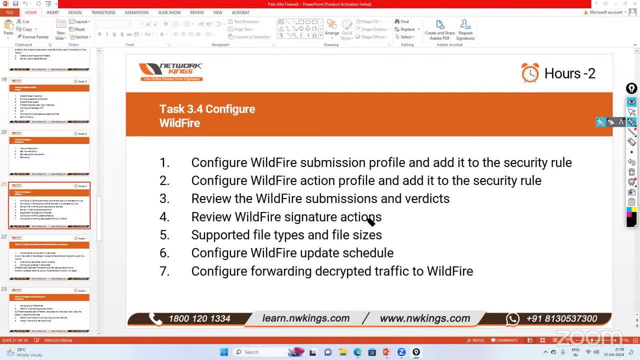 it is analysing it And it sends it to the cloud to analyse it. If it doesn't have any information, that file is correct, By analysing it, it is unable to understand whether that file is correct or not. In that case, 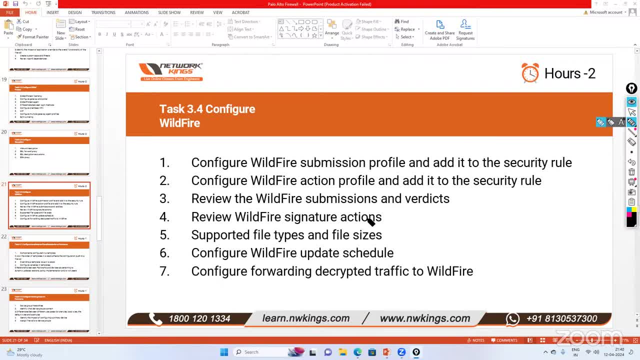 it is sent to the cloud, and cloud will analyse and give you a result saying that we should allow the traffic or we should not allow the traffic. So we have to make sure that the traffic is being controlled. Okay, So it is needed to know. 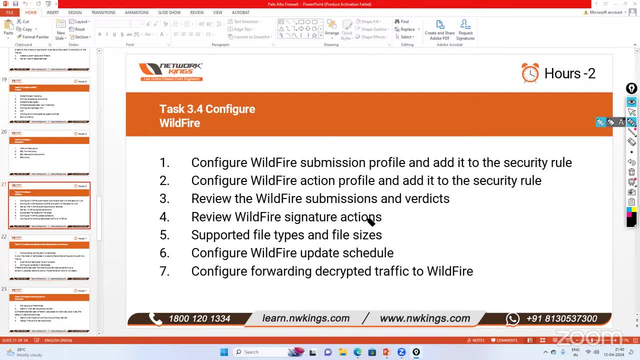 traffic, okay. so wildfire is very much important because there are so many files which is basically infected with malware. there are so many ways we can go or basically open a hole inside the network through this way, so wildfire will help you to protect your network in that particular way, okay. 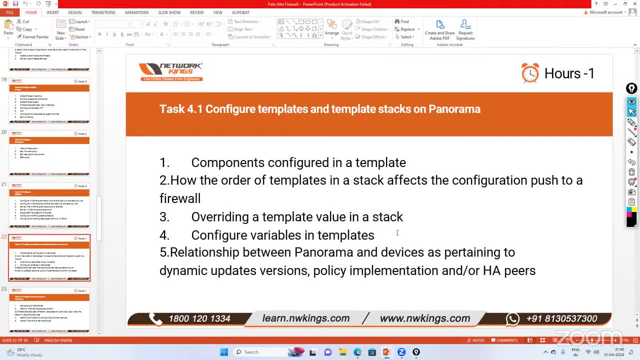 panorama, so panorama, panorama devices so panorama. so our two firewalls here, two firewalls here, so with one interface we manage multiple firewalls. okay, and basically panorama, panorama and we group them, something like that. so we group them. to group them, we need template and device group. 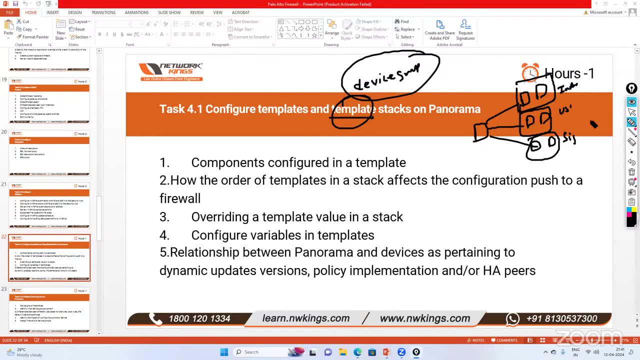 so we group devices of these two ways, because template has some configuration part and device group has some configuration part, and we group them by grouping common configuration. implement it. I will tell you, Then you will understand it better. So what I mean to say is that if I have to manage devices, then it is not. 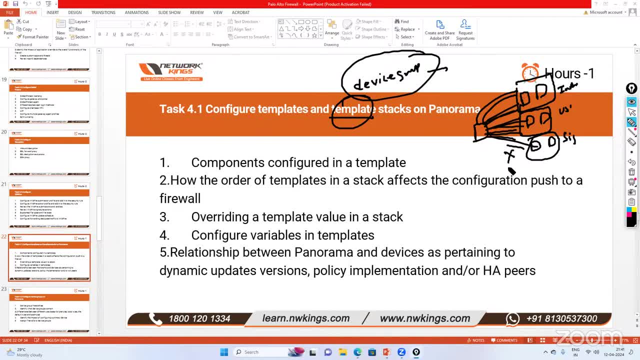 that every rule should be implemented on every device. No, it is not possible, right? So what will we do? We will group it. This is the policy of India. So whenever I will configure it in the Indian group, it will be implemented in the Indian firewall When I will change it in the configuration of the US. 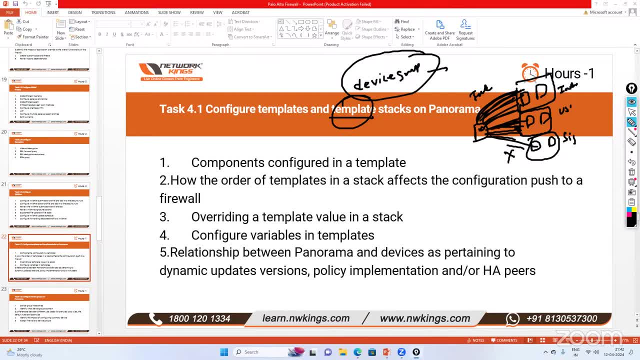 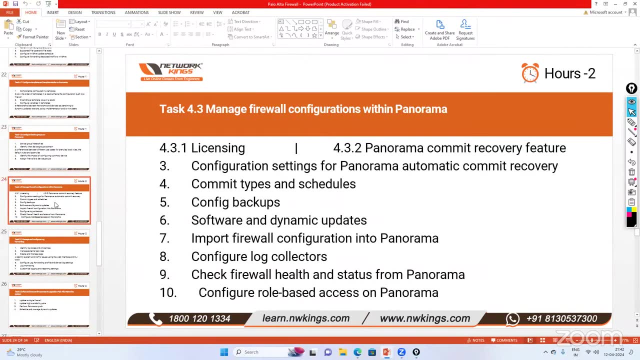 it will be implemented in the USB device, So in this way we can group devices. So there are basically two ways to group: one is a template and the third is a device group. Ok, And we can do a lot of things with Panorama. 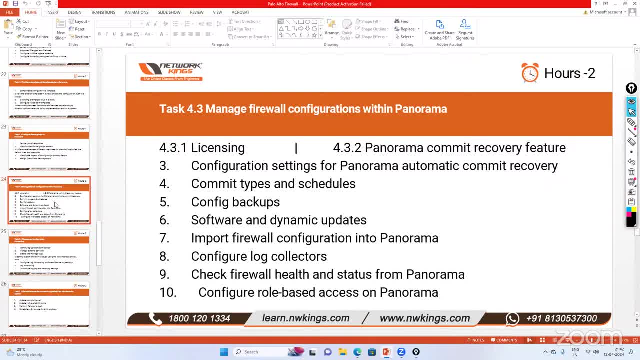 We can commit the configuration, we can take backups, we can take logs, we can upgrade. software means that we can- mostly we can- do everything with firewalls. we can even do troubleshooting. we can receive logs from devices and we can analyze logs. so with one window we can manage all firewalls in every way. 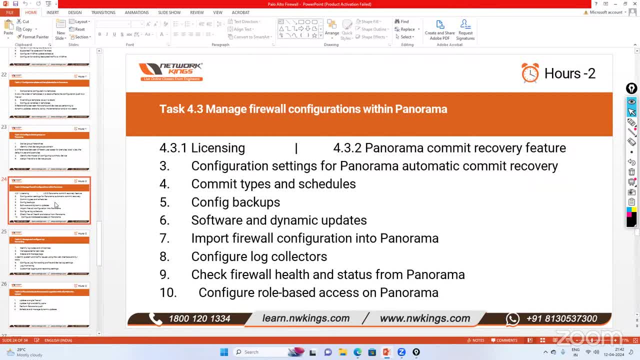 if we want to upgrade, we want to take backup. we want to send updates, like the update of url filtering or update of application control. we want to collect logs. we want to see the health of firewall, what is seek utilization, what is ram utilization- we can see everything. 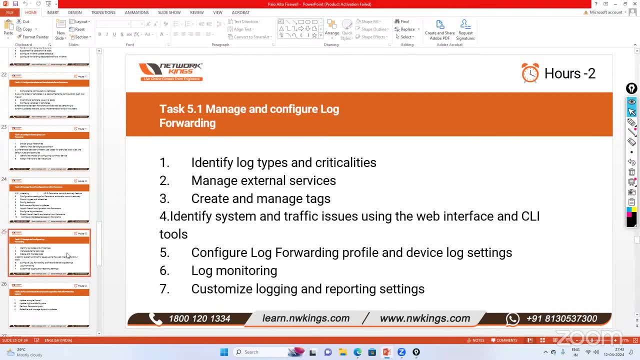 ok, and we basically collect the logs and make a graph of them in a proper way that the users of these devices use facebook more. so, basically, a proper graph is made that this set of users or this set of subnets are going here, this set of so, if you want to make that graph, 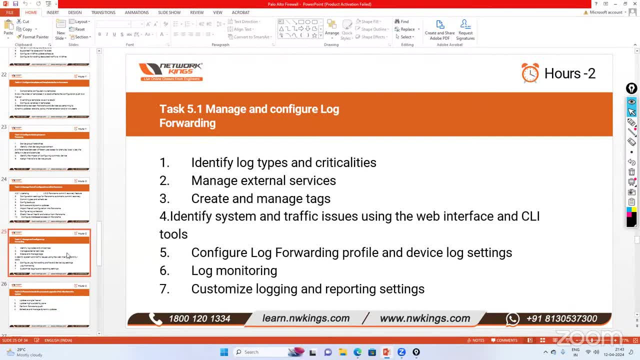 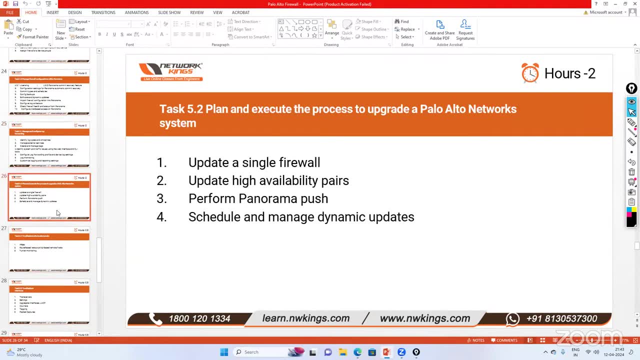 you can do it by setting at panorama. you don't need to log into the firewalls, right, so you can do that as well. we can do many more things through logs. ok, so when we upgrade firewalls, then what is the process of upgrading when they are in HA? 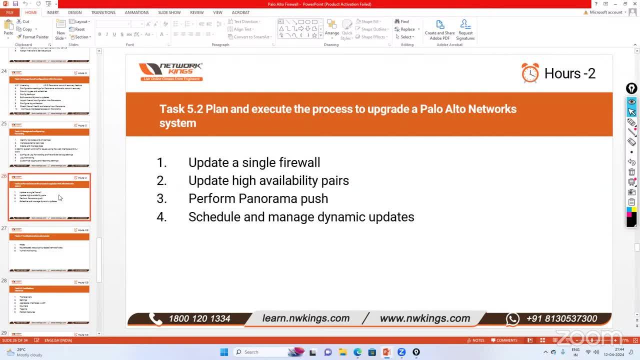 then what is the process when they are in standalone? then how does it happen? how do we push the update through panorama? how do we schedule it right, all these things? we will be covering it now. let's come to troubleshooting. so our firewall topic is over. our panorama topic is over. 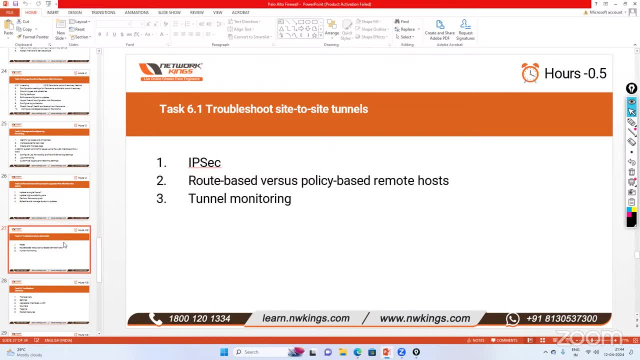 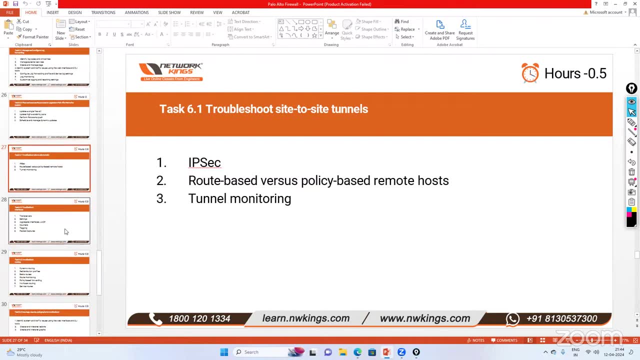 now we come to troubleshooting. so how is IPSec tunnel? what is route based? what is policy based? how do we monitor the tunnel? all these things, ok. after this, how do we troubleshoot? by going to interface base? which information do we check? how do we do packet capture? 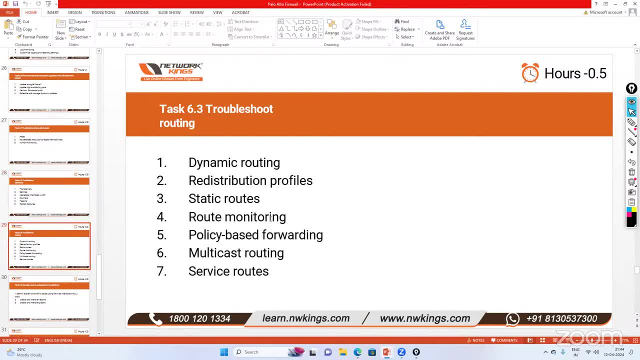 all these things then comes: how do we troubleshoot routing? so routing is basically a very generic topic. so what happens in routing is that if you are actually good in routing, then here through firewall, there is nothing to learn about routing, like if you troubleshoot in OSPF. 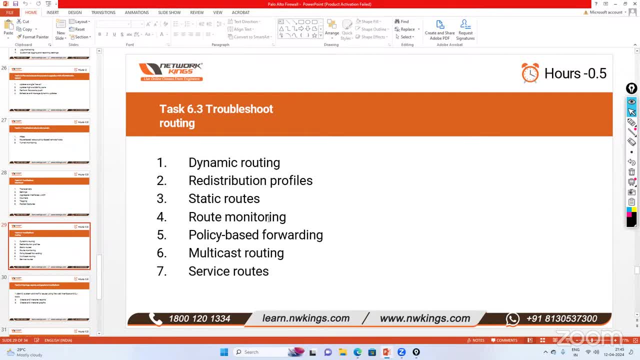 how do you troubleshoot? options are a little different here. you have to check, you have to read that this route is it learning from OSPF or BGP, right? so why is it learning from BGP, OSPF? so you should know how does the routing protocol work? 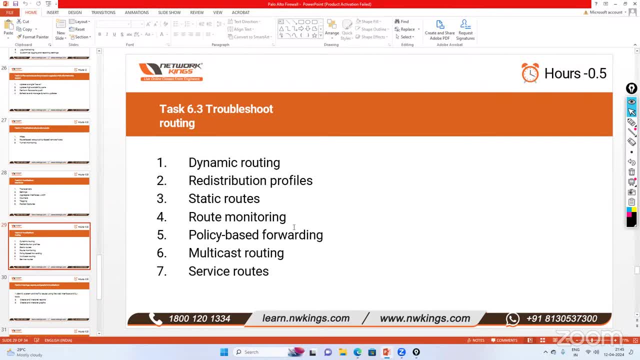 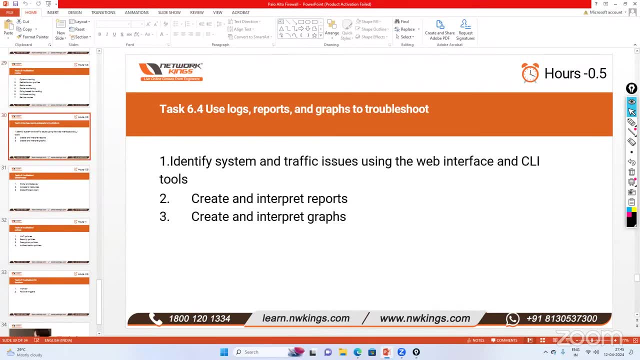 ok, and then we troubleshoot that way. ok, after that same what I told you, that how do we logs like bandwidth utilization is more so we logs, we can take out its report, we can see logs, we can see graphs that at that time bandwidth utilization was, how much bandwidth utilization was. 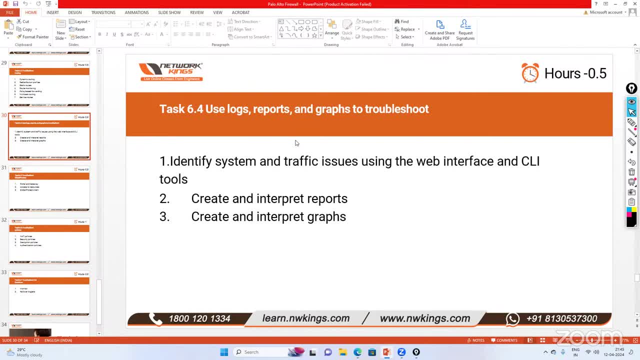 so we can check that way by generating the reports. ok, it is global, like user is not getting connected or user is not getting access. means suppose I am working from home, or if i am connected to my network like VPN, I am unable to connect to or I am unable to connect to VPN. 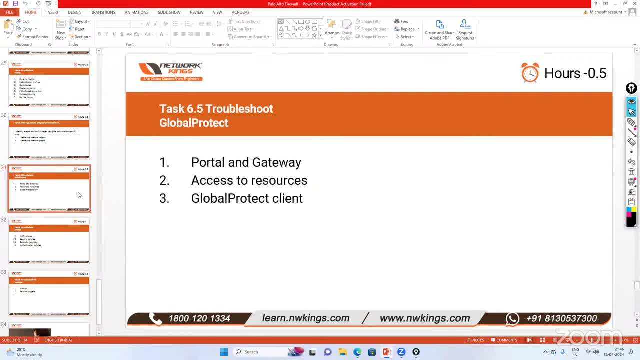 so why is it not getting connected? then how will we troubleshoot if I am unable to access the company resources? so why am i unable to access it? so how to basically troubleshoot that? we will see those things as well. ok, Then how many issues come in? NAT, NAT's, security policies, decryption- so we will troubleshoot all those things like this. we will be seeing that, okay. 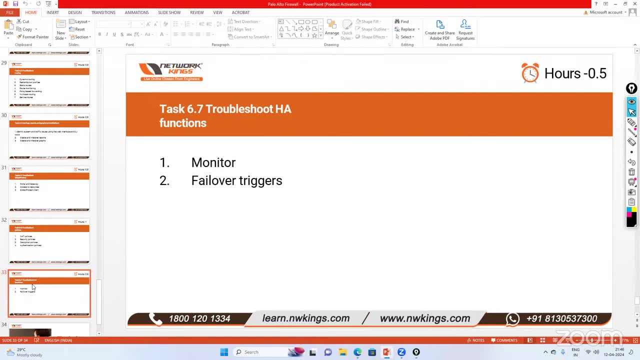 And lastly, when we enable HA, when does failover trigger? when does active- sorry, standby- become active? when does active become standby? what do we monitor? we will see all those things, okay, And after that, my sessions. how does it happen? it is divided into three parts, okay. 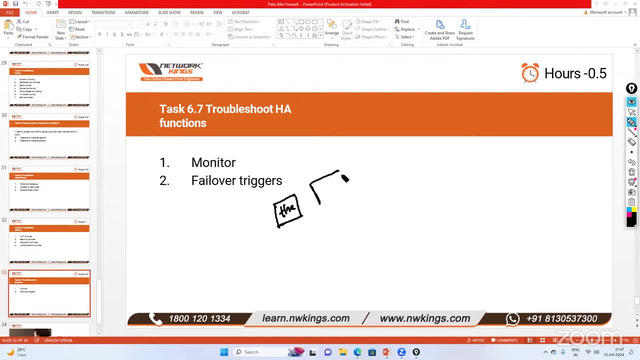 So first of all I cover theory, after that I cover practical, after that I basically include troubleshoot and troubleshoot and my experience is that in practical, when I faced any problem, what issues I resolved and how it was resolved. 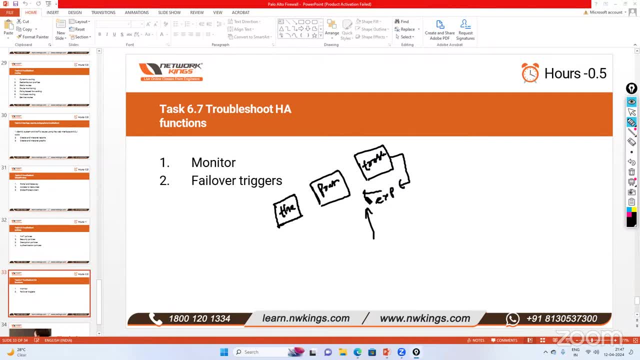 I will also be covering all those things in my sessions as well. So discussions keep happening like this, or I keep telling what happened in my experience, how I did troubleshooting, what things we should see, what things we should not see. so there are a lot of things that you don't need during troubleshooting, but still we consider those things and this makes troubleshooting late. 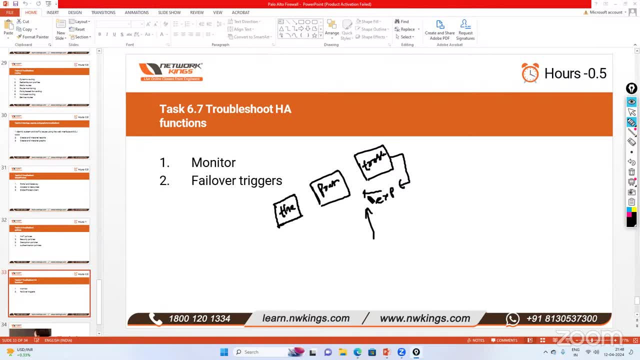 If you have a high priority case, then how can you resolve it quickly? what information you need? I will include all those things. Okay, So I will cover all these topics and I will cover them in this way. okay, The time written here. okay. 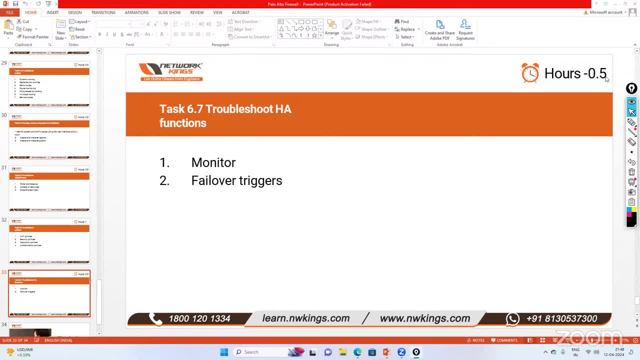 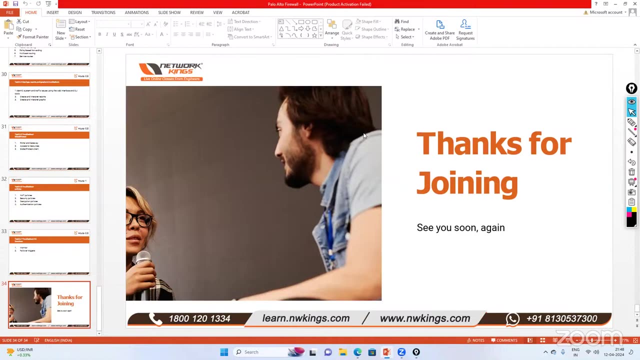 This time is actually only written. Sometimes it is more than this. So if you calculate this thing, then it will actually be less. I will cover more than that, Okay. So this is all about the topics which we are going to cover in this series. 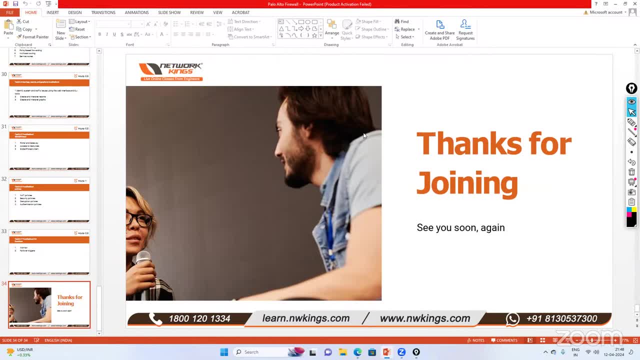 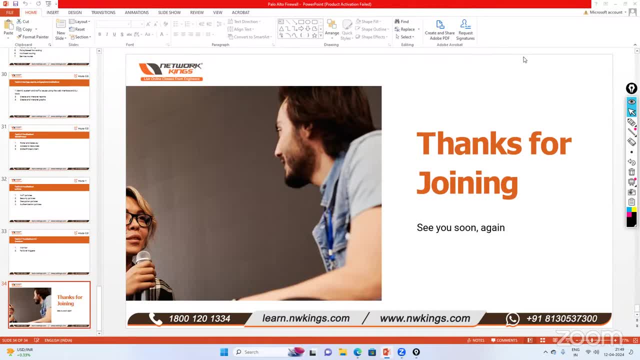 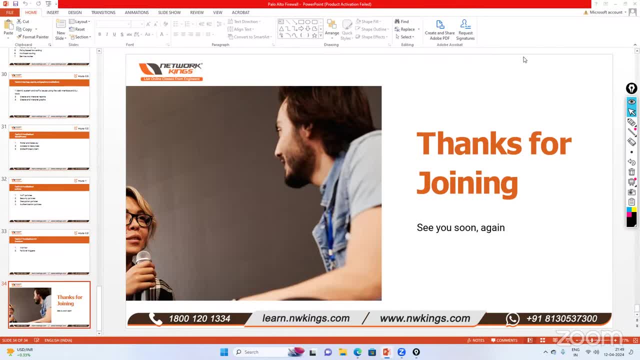 We will use it, we will install Palo Alto on it and we are going to do the packages. Sir, suppose we have access to Ewenji, but suppose we want to do it on a personal device by using that application. can we do that? 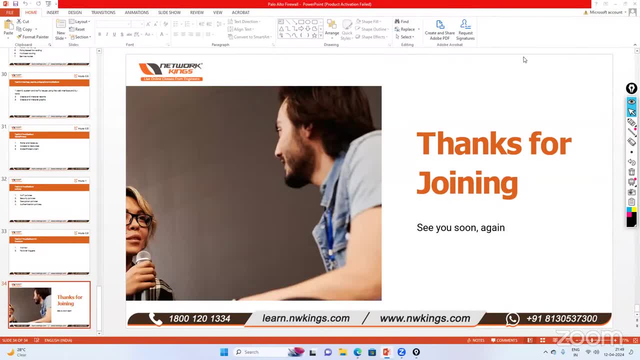 Yes, we can do it. We have a very good, detailed video from Network Kings. I will send you that link. You can easily set up with it. There is no problem, Sir. this is how networking provides access. there is lab access, but suppose? 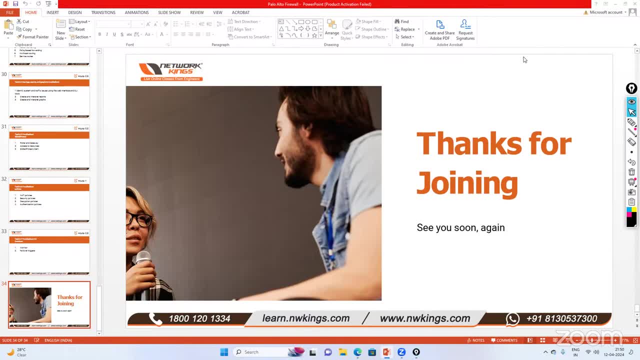 You have to make your own lab on your PC. Yes, sir, It has given steps like that video is made. it has given full steps on which software you have to install, which image you have to install, In what way, what kind of resources are needed. everything is covered in detail. 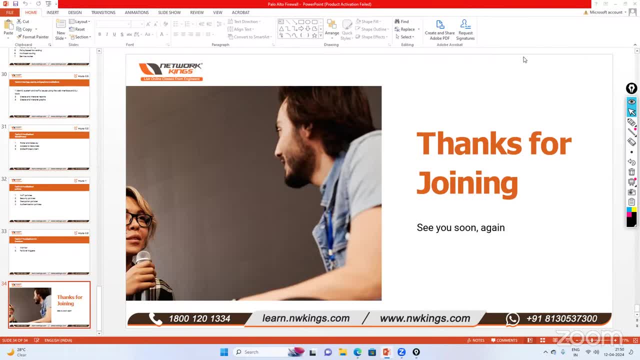 So I will give you a link. you can follow it. Okay, thank you. Can we add you in GNSys? Sorry, sir, I have added him. I have added him in GNSys, the lab I have made. 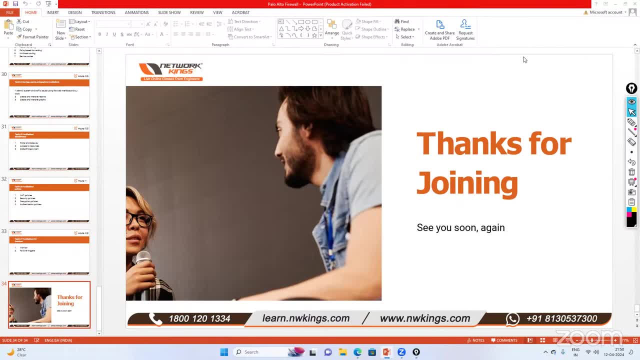 So can we put a photo in it? I actually don't understand the question. Sorry, sir. What are you asking? GNSys, Can you put images in it? I have supported the image of GNSys. Can you put other images? 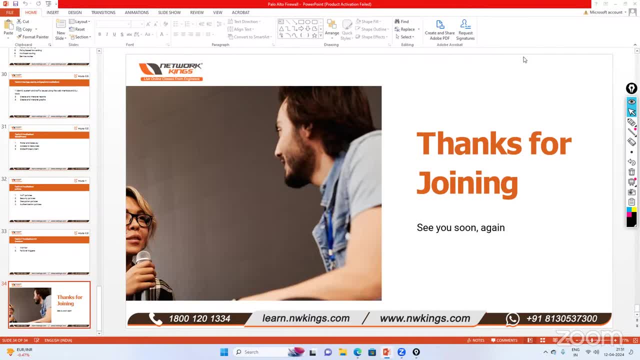 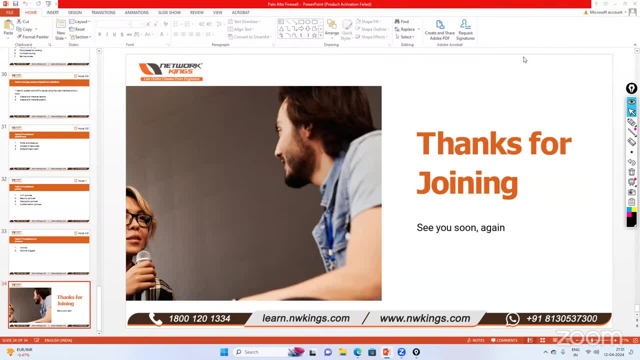 Okay, Sir. do you provide training for Paolo Alto or for FortiGate and Check Point In Networking? actually, right now, I only provide training for Paolo Alto right now. Okay, Okay Sir. the PCNC, is it an ad? 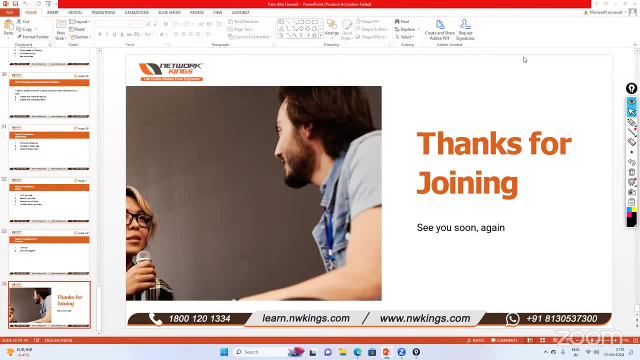 Is it an ad? Yes, So what is an ad? What are the main things in that ad Is an ad. PCNC is an ad, So the two blueprints of PCNC are the same. Apart from that, both panorama and troubleshooting are an added on it. 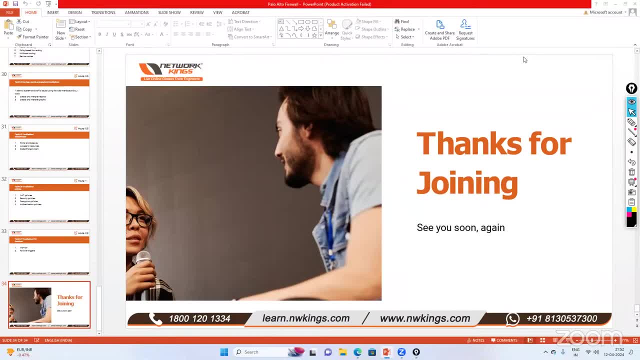 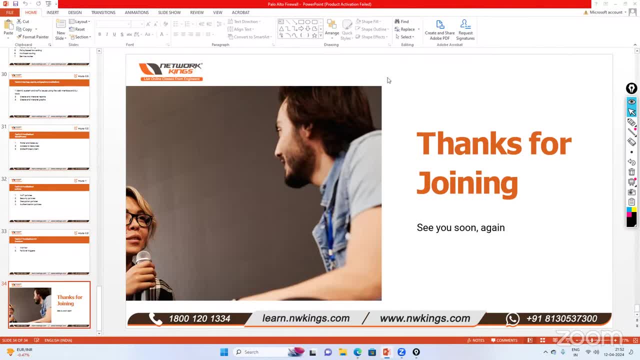